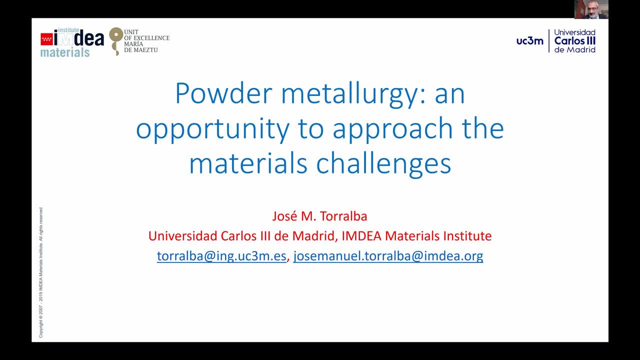 INDEA Materials Institute launches today the first episode of a scientific technological webinar series given by its principal investigators. The aim of these webinars is to disseminate the knowledge we have acquired through the years in order to study, develop and process better materials that can contribute to solutions to societal challenges. In this first webinar, 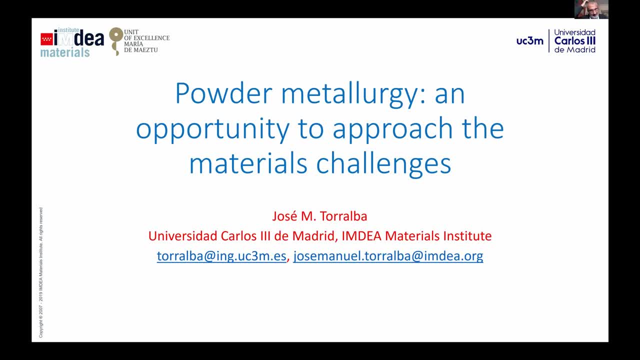 Professor José Manuel Torralba will talk about the importance of the importance of powder metallurgy and the opportunity to approach the materials challenges. And regarding the structure of the webinar, it's going to be organized in two main parts. The first one is obviously the most important one. It will be the talk of Professor Torralba More. 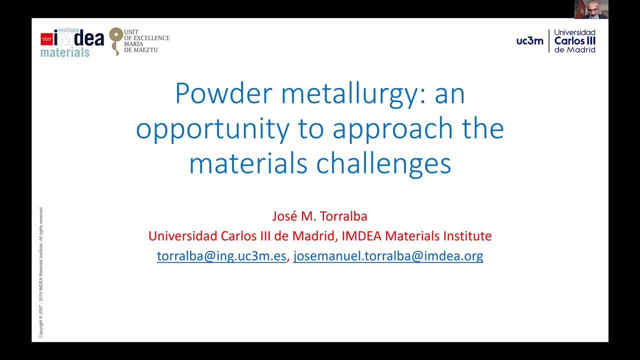 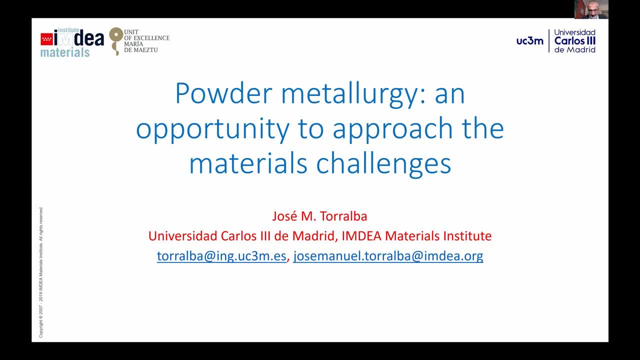 of discussion, And then we will have another 15, 30 minutes for open questions. So visit that. I would like to, And before I start in the webinar, I would like to introduce a today's speaker. As everyone knows, he's Professor José Manuel Torralba is. He's a. 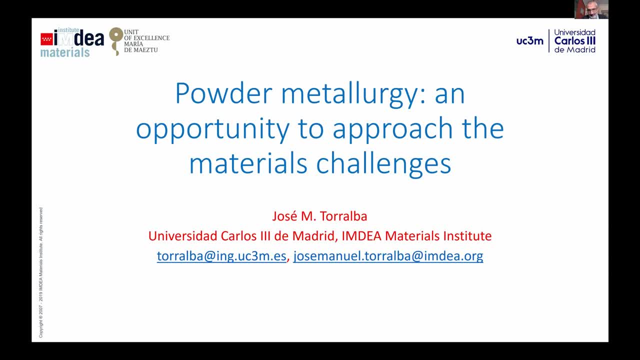 fully professor of materials science and engineering at the University Carlos III of Madrid And also a senior researcher at the INDEA Materials Institute, where he's master of Scottsdale, currently leading the solid state processing R&D group. and a short summary of his long career and successful career. I would like to mention that the well he 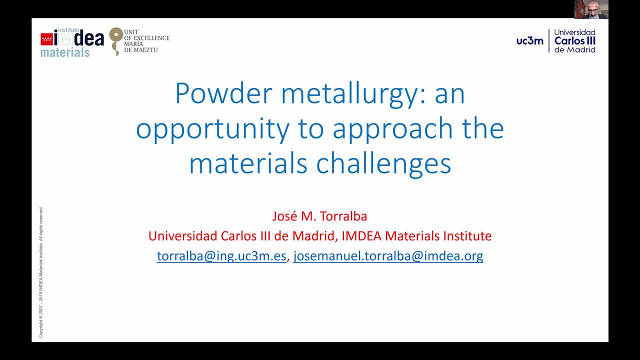 has been head of the material science and engineering department at the Carlos University of Madrid. in 1999 and 2000 he was also vice-rector for academics infrastructure university. from 2000 to 2004 he was also vice rector for research- an innovation, Carlos, I tello- the University of Madrid as well. 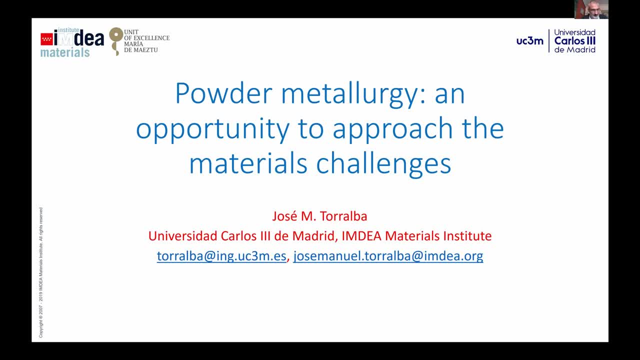 from 2004 to 2006, deputy director at the institute in their materials from 2009 and 2015, and then from July 2015 till August 2019, he was the general director for universities, research and higher administration and administration Artistic Schools of the Madrid Regional Government, His main scientific and technical field of. 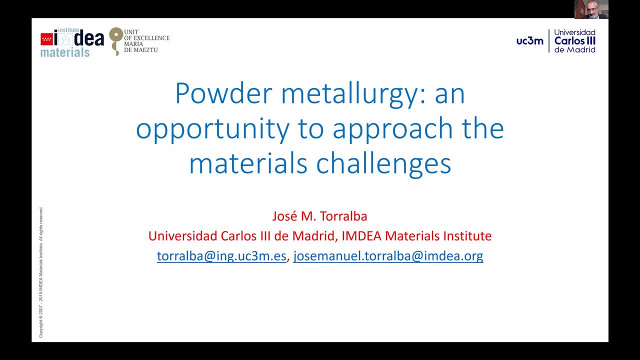 interest is powder metallurgy. He has published more than 500 scientific papers, 250 of them in the GCR index, with more than 5000 citations, and he has supervised 29 PhD theses and 90 diploma theses. He has participated in more than 70 international scientific committees of 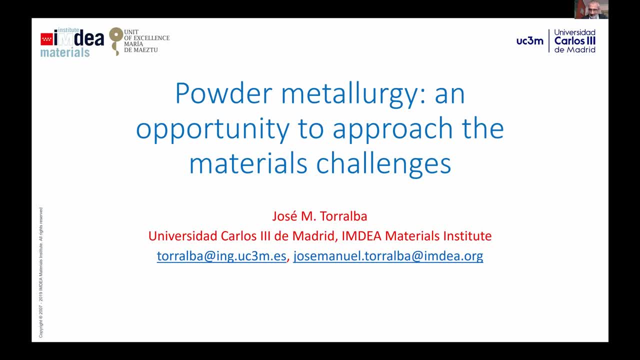 international conferences and being chairman of seven of them, including AMTP 2001 and AMTP 2015,. has been involved in 35 competitive projects in regional, national and international frameworks, being main researcher in 25 of them. has managed several research grants and contracts with. 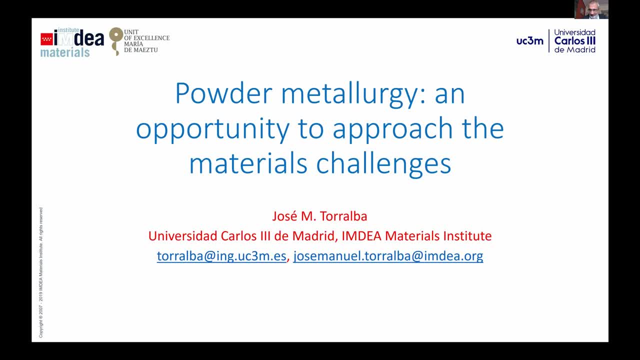 industries and has been a leading researcher in the research and development of research projects. He is a regional editor for Europe of the Journal of Materials Processing Technology and Metals, and he is also editor-in-chief co-editor of Powder Metallurgy from 2009 to 2015,. academic supervisor. 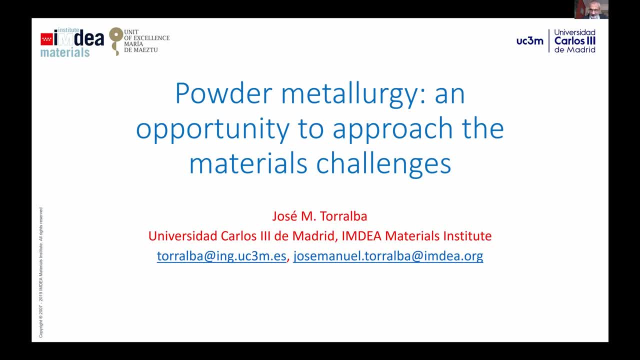 of the EEBMA Summer School. I could actually add a lot more things about the successful career of Professor Torralba, But well, what we want to really hear today is his technical expertise and all the things that he has to tell us about powder metallurgy. So with this, I would like to give the word to 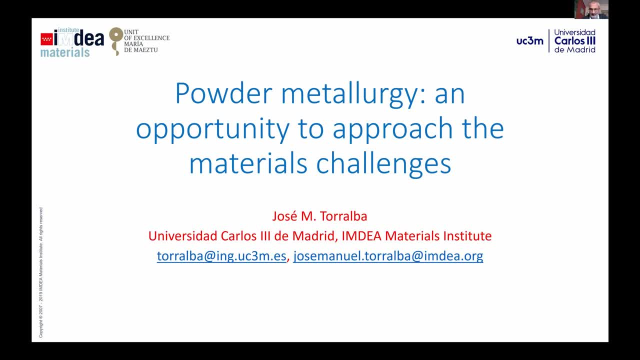 Professor Torralba. So please, whenever you want. Okay, Miguel Ángel, thank you very much for your kind introduction, and let me just start to give the thank you to the people who have joined us today. I hope that with this webinar, we will. 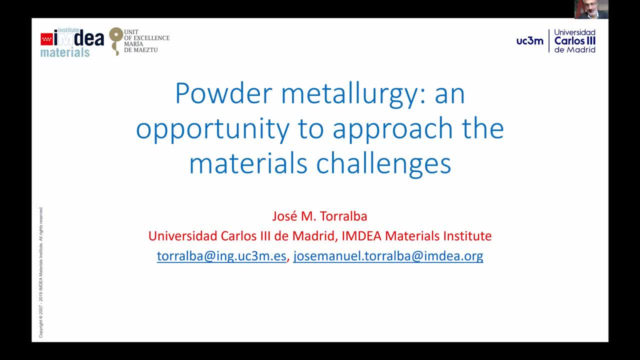 help the people in this difficult moment that we are living in Spain and in other countries. I hope you will enjoy this talk and also I want to say that this general is a talk structure in order to have a divulgative objective. So for those of you that I have seen, 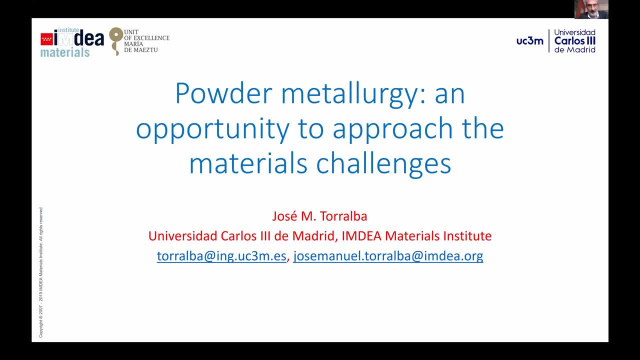 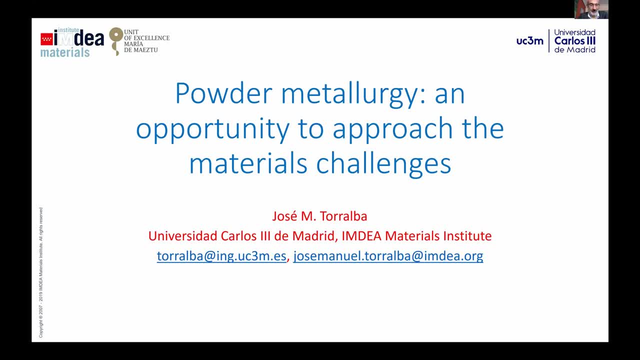 Thank you, Thank you, Thank you, you too much- and to give you some new ideas and open new windows. anyway, also, i want to thanks to india to be the first in this webinar series. that, i think, is a very nice idea and for me it's really. 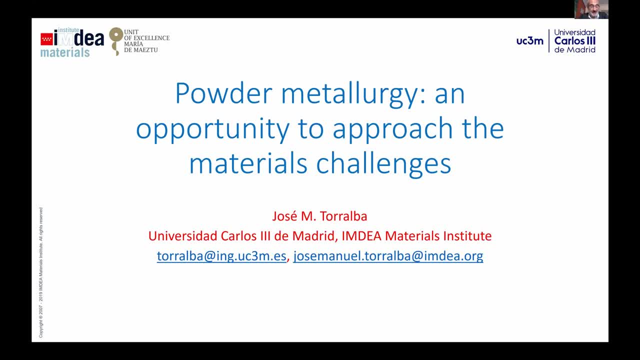 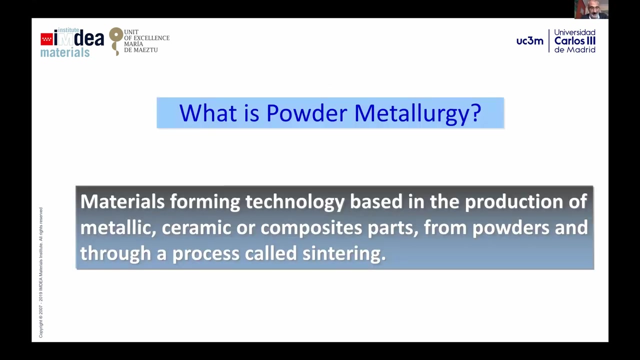 an honor to start with this series and especially because i am going to talk about powder metallurgy as an opportunity to approach the material challenge, because powder metallurgy has been the core of my activity, my professor and researcher, and i am really happy to talk about this, this topic. so let me start just defining what is power metallurgy, because, uh, from the beginning, 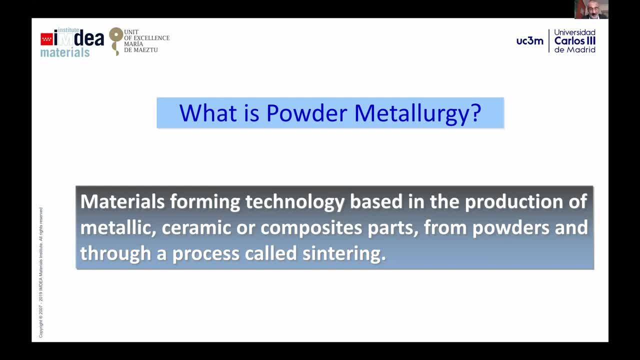 we have to say that powder is a positive performing materials forming technology which is based in the production of composites, ceramics and metallic part. when we mention the word metallurgy, we are thinking especially metals, but metallic powders can be mixed with ceramic or other kind of powders and with this technology we go from the powder. 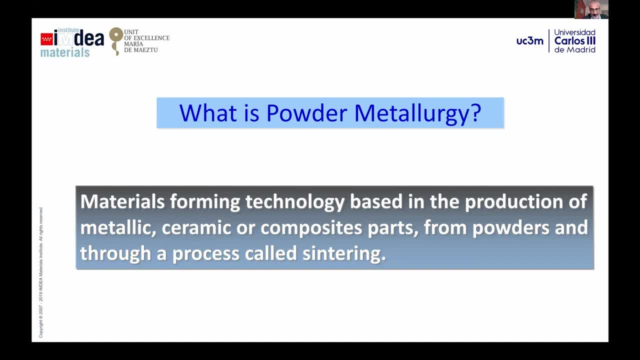 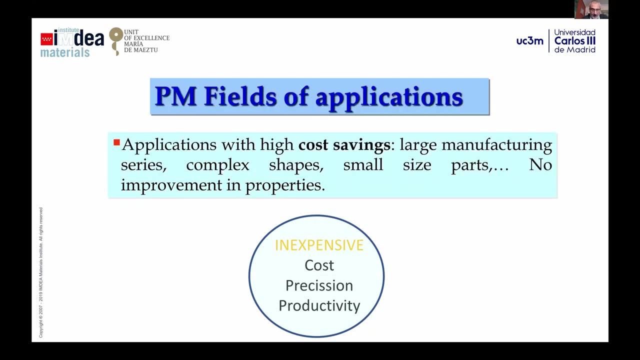 to the part through a process in which in the core part is the sintering process, which is the part in which we get the more percentage of the final properties of the material. we have different fields of application for powder metallurgy. the first one is the most known- is the application. 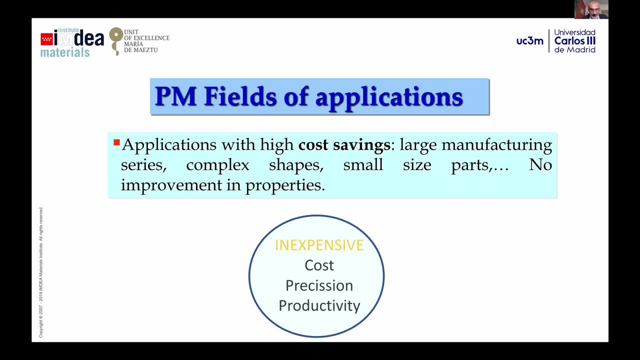 in which we have a high level of cost savings. in this case we are developing cheap materials, cheap parts. that means usually large manufacturing series, complex shapes, small size parts. but one characteristic of this field of application is that usually the properties that we have at the end of the process are not so good as in another. 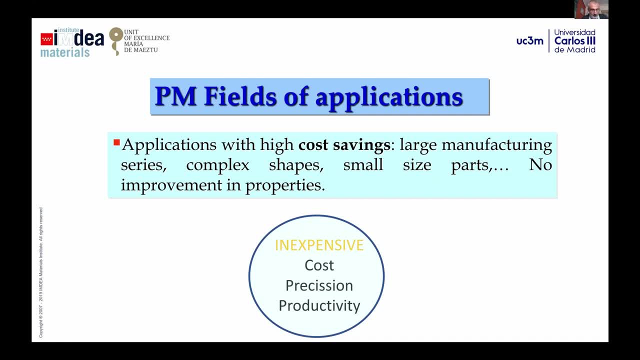 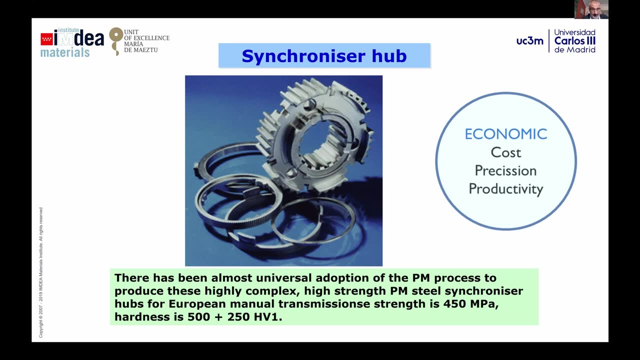 alternative processing methods. so the main value of this field of application of powder metallurgy usually is the cost. one example of this of this field of application is the synchronizer hub. synchronization hub is a very interesting part. is part of the transmission of one conventional curve and in one in each transmission. you have at least five of these synchronizer hubs and this part. 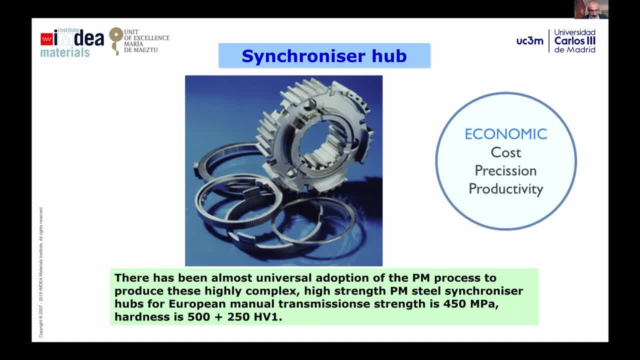 usually were made in the past, maybe 20 or 50, more than 15. 20 years ago it was made by 49 machining and this part by this alternative and, as i mentioned earlier, it's a very, very significant obligation. so this is the only future that this we are doing now. 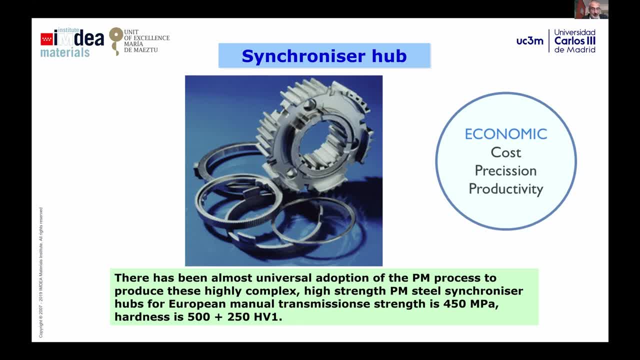 So for this particular work is the synchronizer hub, and we have five types of this synchronizer hub. alternative method: by forging and machining. the cost to develop this part is in the order of 40-50% more than by powder metallurgy. 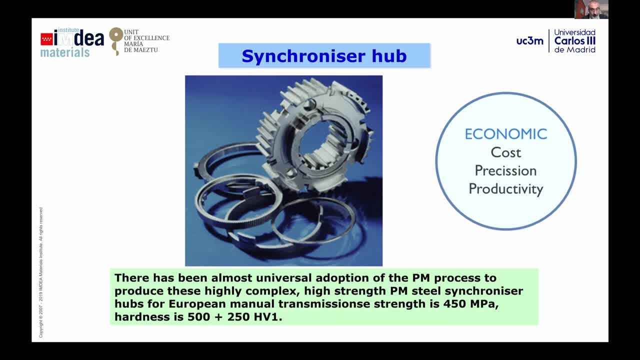 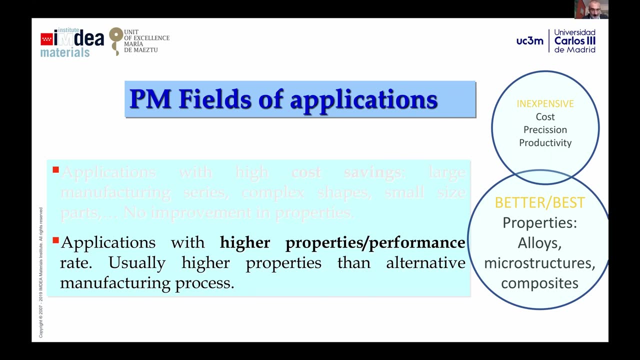 By powder metallurgy, you can develop the part with enough properties to fulfill the requirements of the transmission of the car, and at much lower price. If we go to the second field of application, it is the completely opposite field of application. In this case, through powder metallurgy, we can produce parts with much better properties. 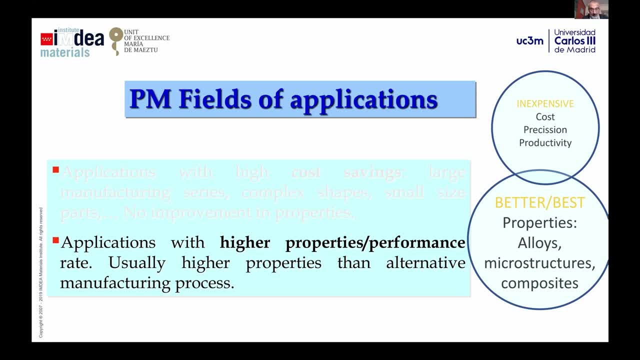 than any other alternative manufacturing process. Why? Because powder metallurgy can assure by different ways a better microstructural control, a better chemical control of the composition, no segregations and a lot of different things that can improve a lot the properties. 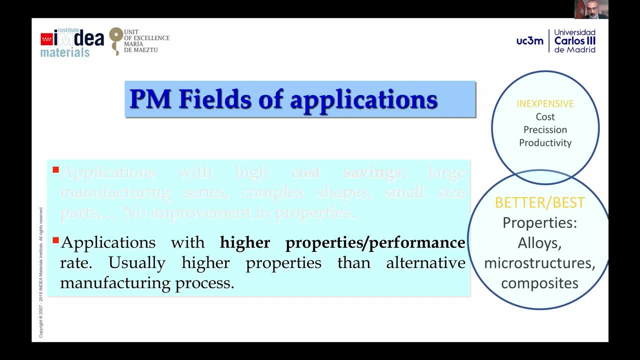 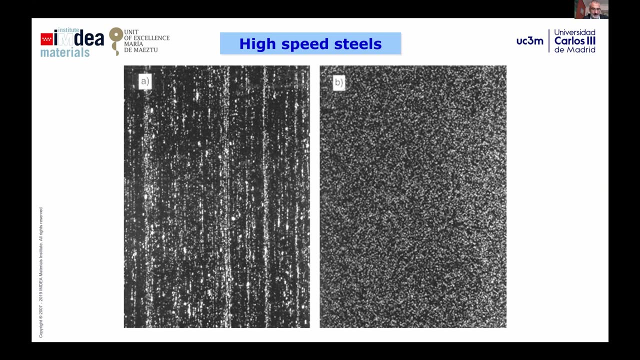 In that case, powder metallurgy is the best way to obtain one determined part. One example of this field of application is high-speed steels. High-speed steels can be produced by different ways: By casting, forging, of course, and then machining, and so on. 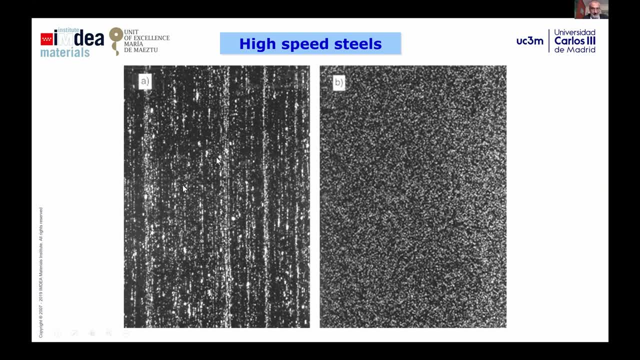 On the left we have a typical forged high-speed steels. If you see the microstructure you can see in the matrix of iron, of iron-based material, you have a lot of black, sorry, the white part of the microstructure are the dispersant. 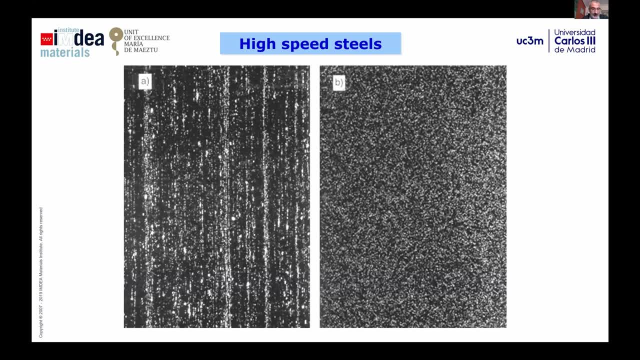 carbides After forging. we have a directionality of these carbides. The size of the carbides are really high And if you compare all of these carbides you can see that the dispersant carbides are very high On the right with the powder metallurgy microstructure. here on the right you have much lower size. 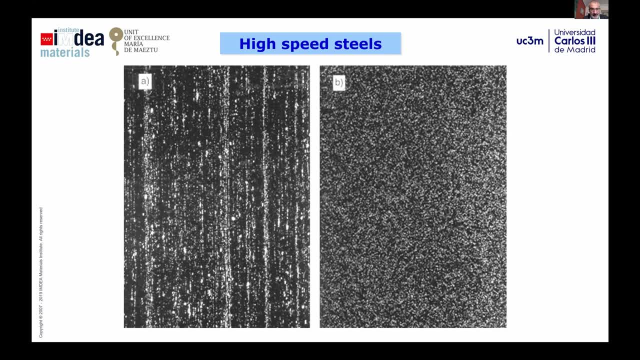 of the carbides much better distributed without any directionality of the carbides. All these microstructural features allows that this kind of high-speed steel produced by powder metallurgy is much better in properties than any other produced by forging or other alternatives. So this is the case of the second niche, the second field of application. 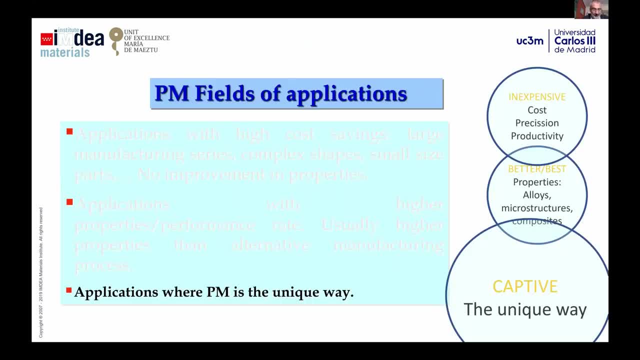 And we can go to the third one. The third one is the captive way. In this way- powder metallurgy- we can say that this is the unique way to produce one specific part, one specific material. So in that sense there is no other alternative. 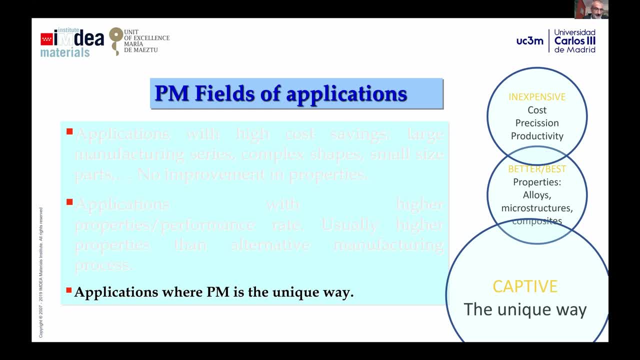 It's not a matter of price, it's not a matter of properties, it's just a matter of opportunity. It's the unique way to obtain one specific part, And we have one example of this also here is the cemented carbides. 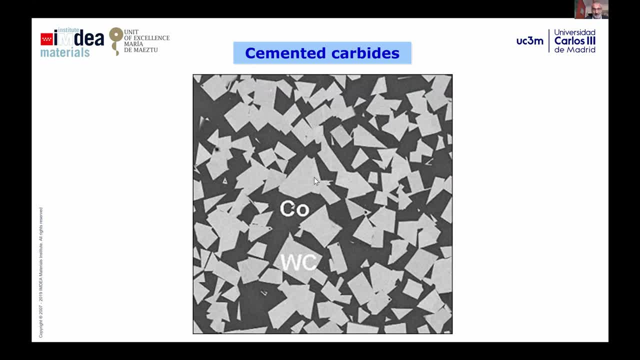 This microstructure that we have on the screen. you have seen a matrix of cobalt with the reinforcement of tungsten carbide And we have this specific microstructure. And with this specific microstructure we have some specific properties that allow this material to have the main part in the market for the cutting materials in the world. 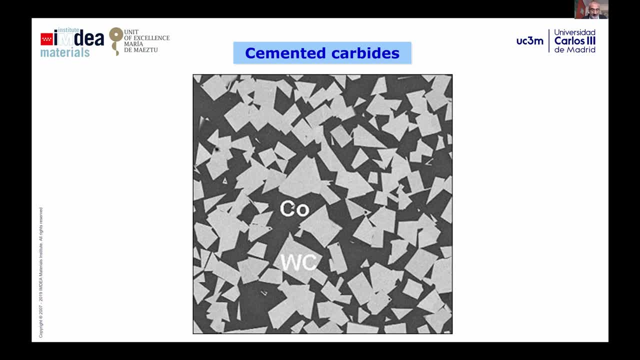 That means that other metallurgy can produce this specific microstructure. You can, of course, you can take cobalt and tungsten and carbon, cast it and to have a material produced by casting or other alternatives. but never you will have such a specific microstructure that can allow to us to. 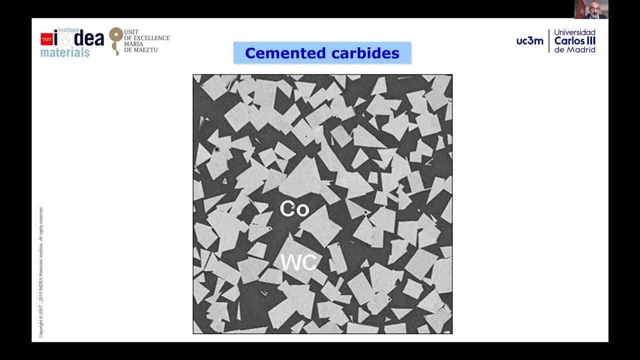 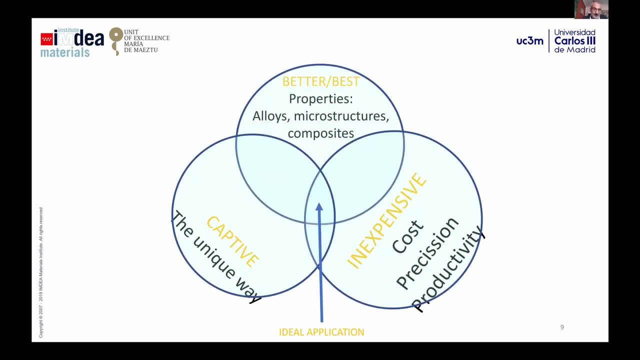 have a wood cutting performance. so this is one example in which powder metallurgy is the unique way to produce one specific material. of course, we can find some applications in which we can combine the three fields of application. we have some applications in which you can, by powder metallurgy, you produce the 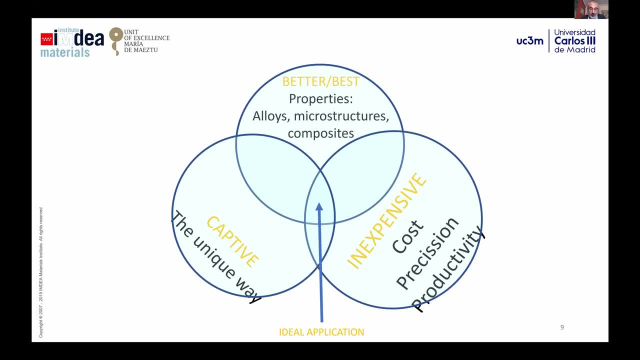 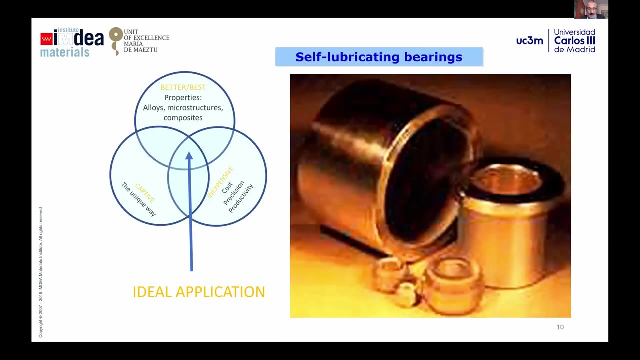 part at lower price. this is the unique way to produce some specific parts, and by powder metallurgy you produce the better material that can be obtained for the for some specific application, and this is one example which is quite well known, which is the self lubricating bearings. the self lubricating bearings, the 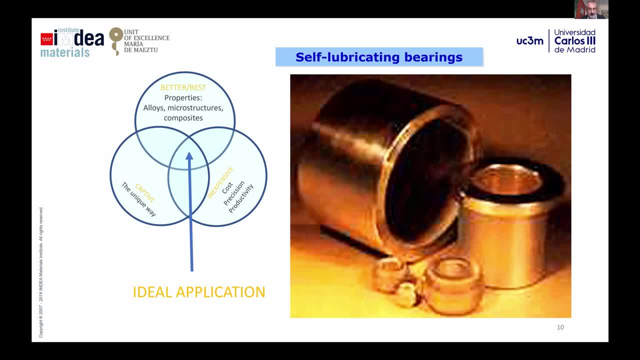 unique way to produce this kind of material is by powder metallurgy, because you have a porous material with some specific porosity, with some properties. the way to produce that is press and sinter, which is the most cheaper way to produce such a kind of part, and by powder metallurgy you can get the better possible properties for this. 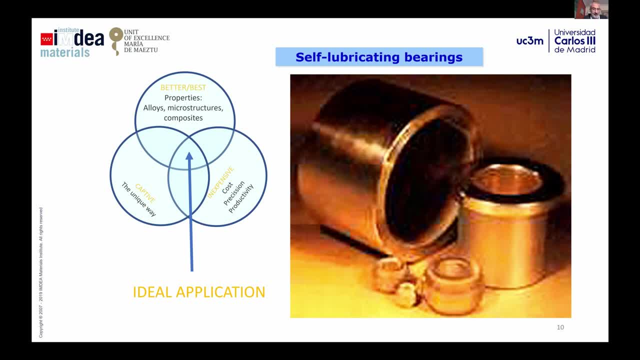 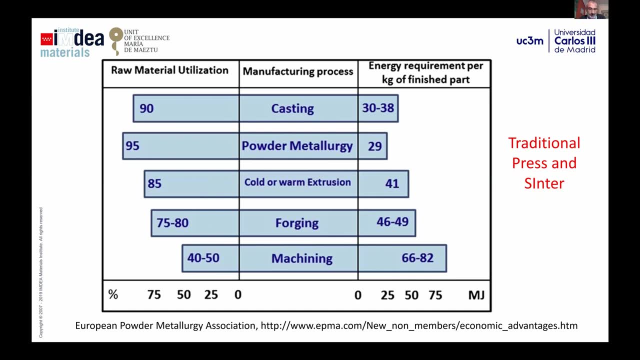 specific application. so this is the ideal application in powder metallurgy. if we go to the conventional press and sinter method, which is the 90% maybe of the parts produced in the world by powder metallurgy. why we have cheaper, cheaper prices, why we have the cost-effective production method, the main. 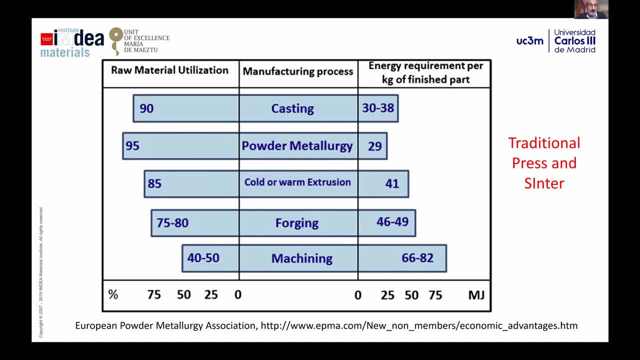 reason is that we use in the order of 95% of the raw material. we don't have any losses in materials or a few losses, and we spend the lower amount of energy to produce a final finishes part if we compare it with casting or extrusion or 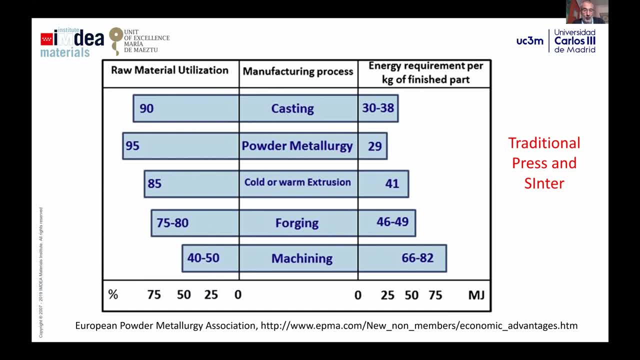 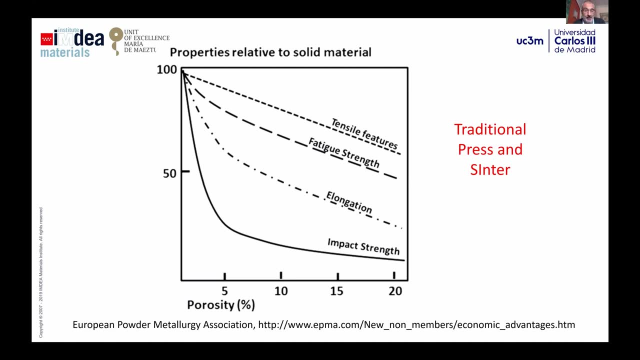 forging or machining. so we are combining low, a low cost of in energy with the high level of raw material utilization. in that way we used to have lower prices and but we have a in the negative part of these of this kind of production method that use we 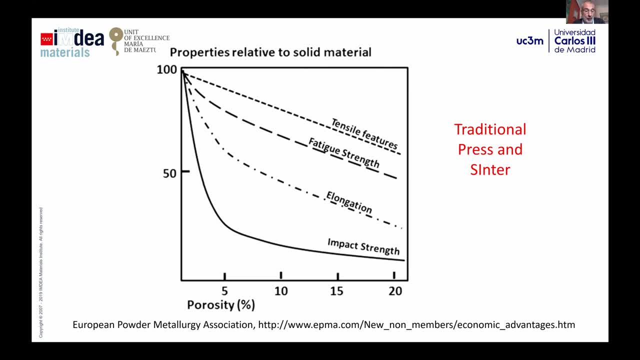 used to produce part with a lot of porosity and porosity decrease a lot most of the properties. of course the tensile fetus are decreasing in a linear way, but if we go to properties link it to the utility of a material such as elongation or impact strength, we will decrease in an exposure in an exponential. 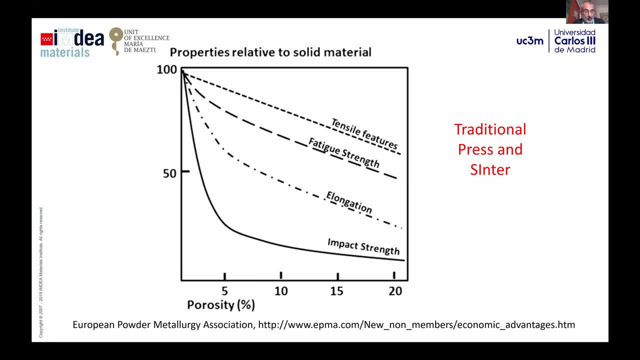 way the properties. just with 5% of porosity in a part we can decrease more, more than 50% of the final property of the material. So that is the typical conventional powder metallurgy in which we have a low cost part with enough. 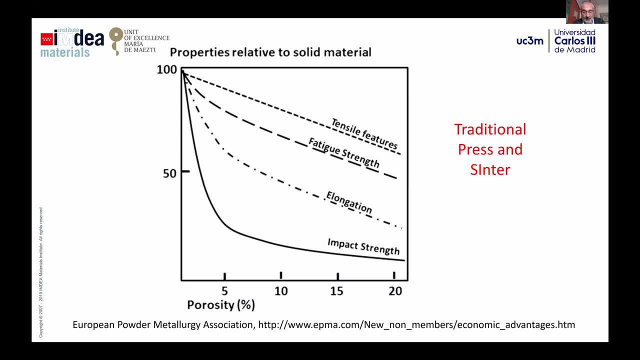 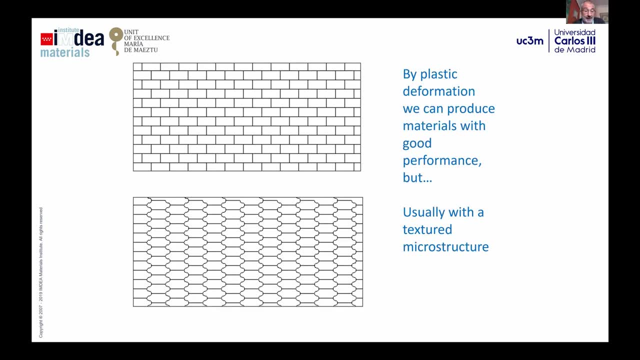 properties for the application, but with much worse properties than the conventional ingot metallurgy or So in general, if we want to compare powder metallurgy with the conventional plastic deformation methods, in plastic deformation methods we have a simulation of a microstructure. 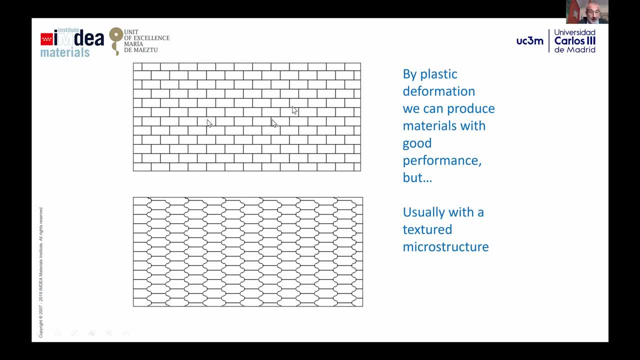 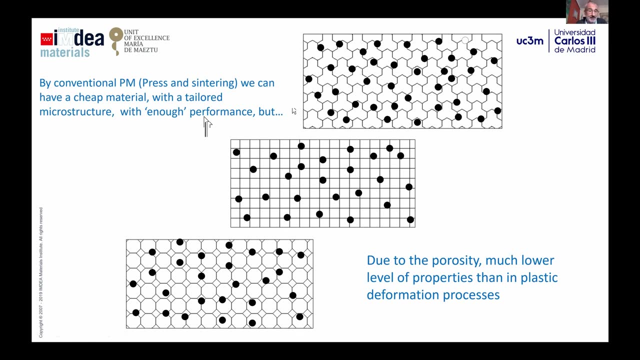 Here you have a texture material, usually without any porosity, with low level of defects, but with a texture microstructure. If we go to powder metallurgy, here we have these black dots simulating the porosity, But by conventional powder metallurgy. 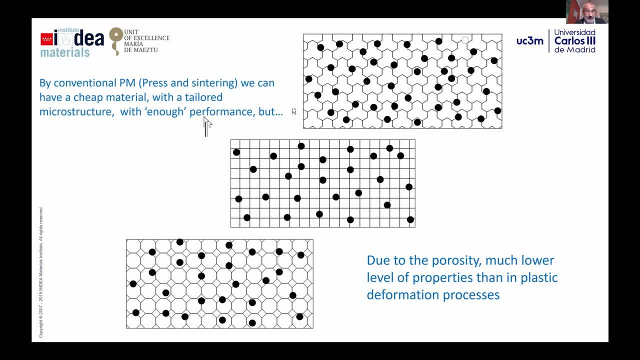 by press and sintering. we have enough performance to fulfill the application that we are looking for, But we have a lot of porosity. That means lower level of properties than in the conventional plastic deformation process. So we can compare on the left the typical microstructure. 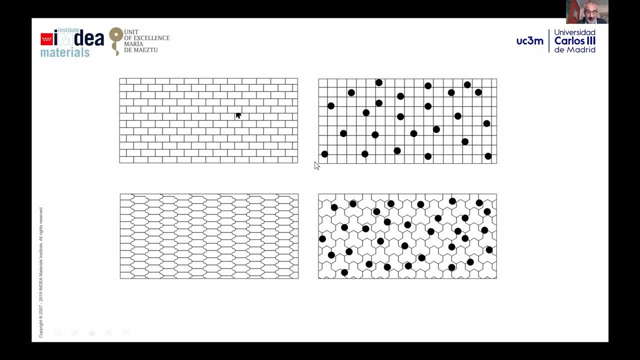 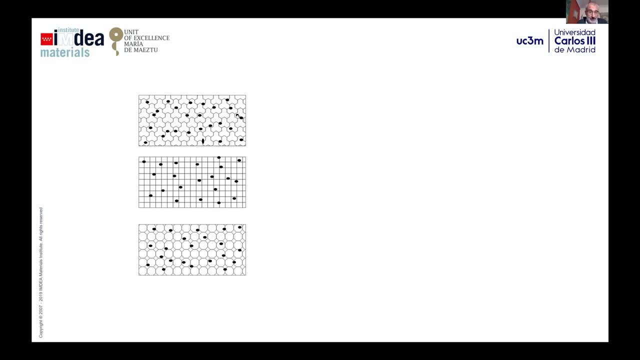 that we can have in a plastic deformation process and on the right, the conventional power metallurgy microstructure obtained by press and sintering. But of course, during this lecture I will try to show you some methods in which we can get. 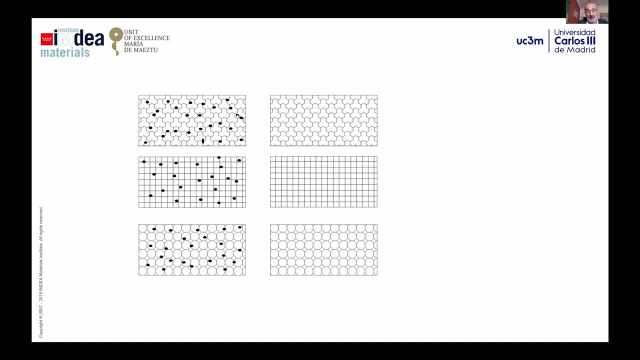 a lower level of porosity. using powder metallurgy We can go from this situation to that one in which we have a non texture microstructure, but without porosity, Or even we can get microstructures with a grain size much more reduced than in conventional even material. 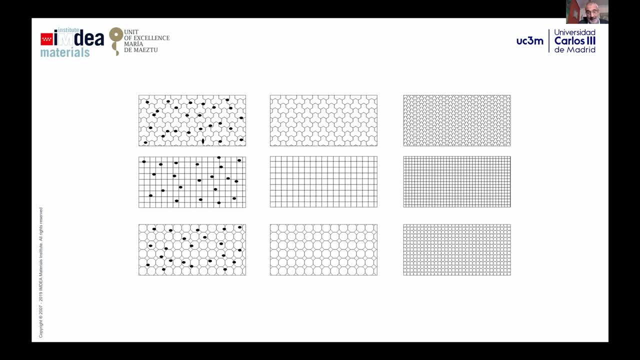 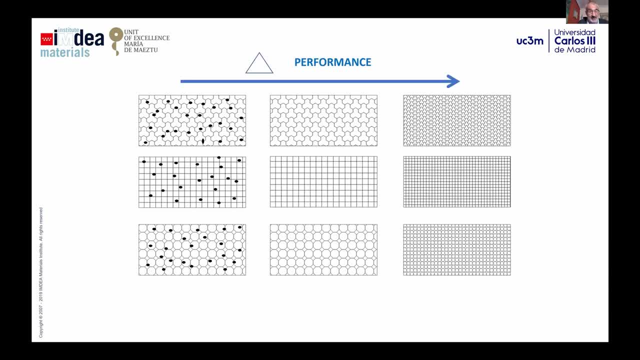 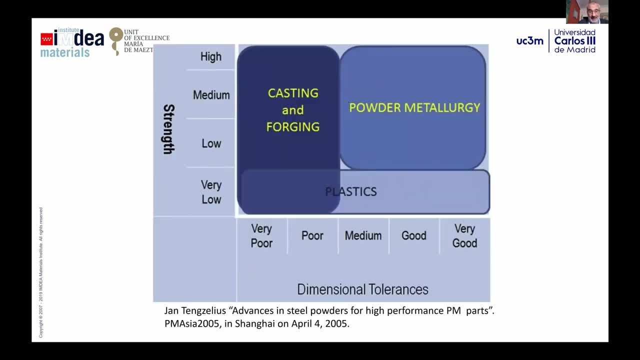 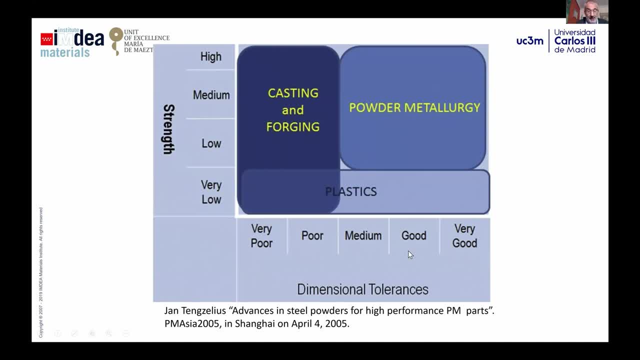 because the dimensional tolerance is one of the advantages of the conventional powder metallurgy. But the level of properties in between the lower level and the high level is highly linked to the way in which we obtain the powder metallurgy parts. If we go to press and sintering, we will have the materials in this side of the map in which we have high level of dimensional tolerance but low level of strength. 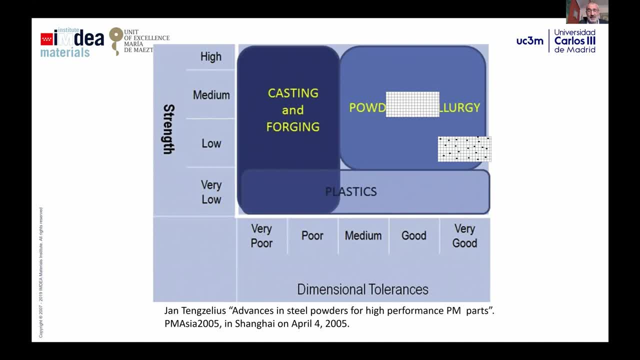 If we increase the processing methods and we go to lower level of porosity, we move in this direction and even we can reach high level of strength with medium-poor dimensional tolerances. but these materials can compete with any other material in other, alternative processing techniques. 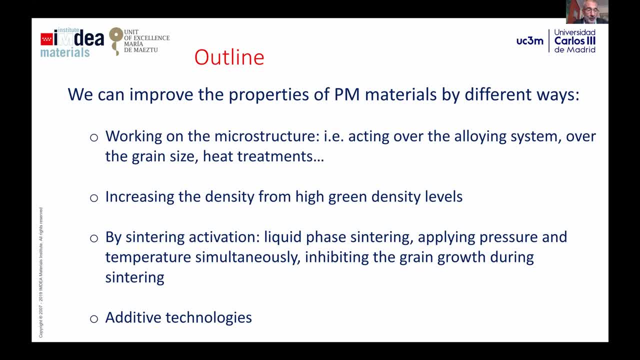 So in this lecture I will try to show you some ways in which we can improve the properties of the conventional powder methanergy materials by different ways. I don't have time to go through in detail through all of them, but I will try to put some examples regarding how we can work on the microstructure. 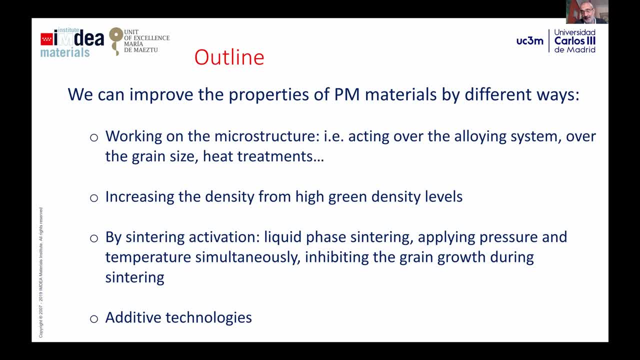 and in that sense we can act over different parts of the processing method in order to produce better properties. We have another way to do this. To increase the properties is just increasing the density from high levels of green density. We don't have time to talk about that, but it's another interesting way. 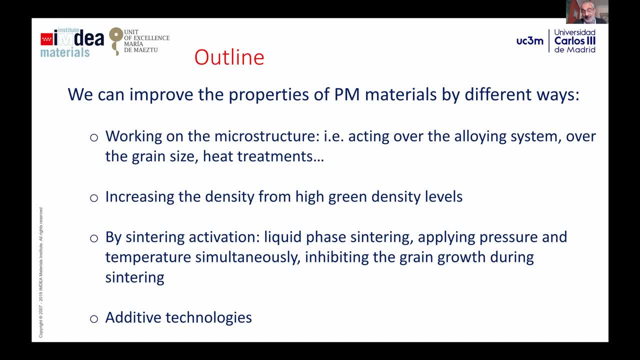 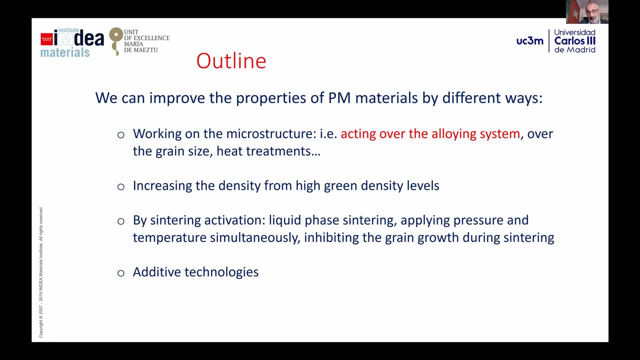 Of course, we can increase the properties by sintering activation, by different ways. I will put some examples in this field. And of course, today we have another completely new field which is really interesting, which are the additive technologies. So, regarding the first of the topics, we can act over the dilution system. 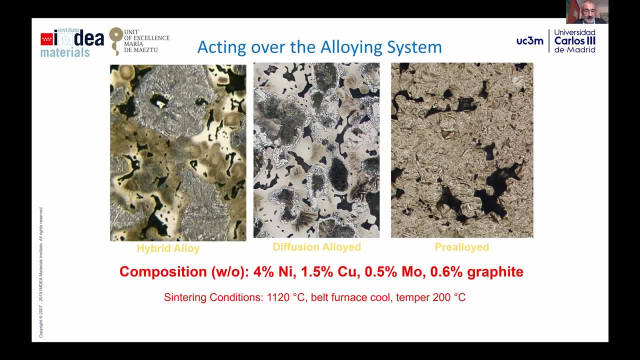 Just to show you one example, Here we have one steel, one conventional PM steel, with nickel, copper, moly and graphite, And with some specific conditions, in that this condition is 1120 degrees, cooling at the furnace and then tempered, And you see that we can have three completely different. sorry, this is the fixed telephone. 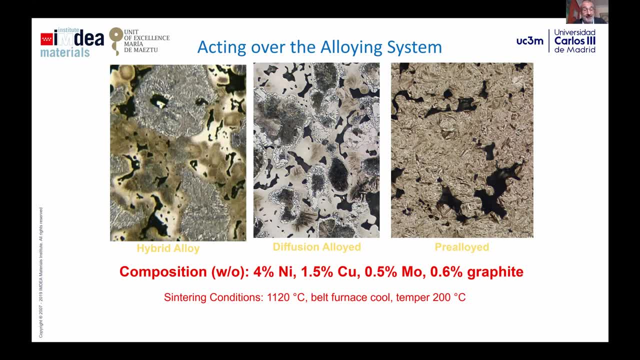 Three completely different microstructures And depending on the microstructure, we will have different properties. And these microstructures can be obtained depending on the way in which we treat the powders: the original powders, So hybrid alloys, or diffusion of allogeneic powders, or fully pre-alloyed powders. 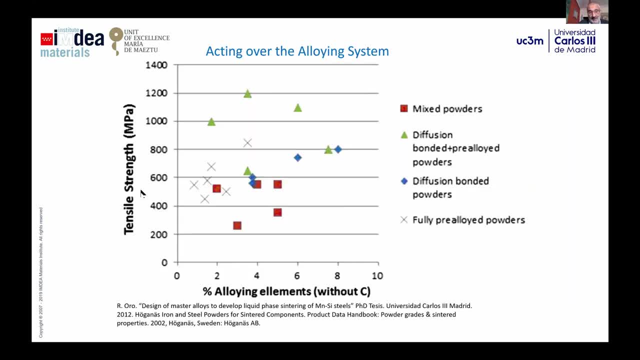 If we go to the properties you see here and we can represent the tensile strength as a function of the allogeneic elements. With the same level of allogeneic elements, for instance, you can go to 4% or 6%. 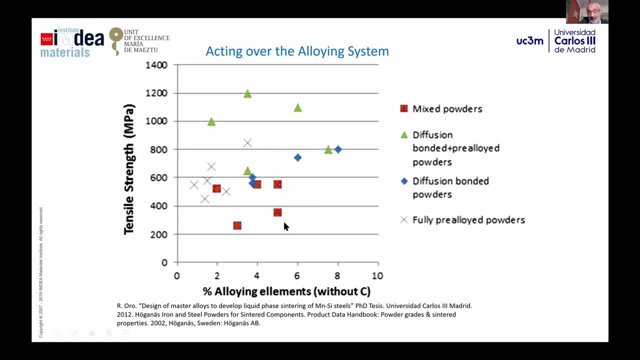 You can have different levels of tensile strength, just changing the way in which you use the powders before starting the process. If you use mixed powders, you go to the lower level of properties. You can go to diffusion-bounded powders and you increase the properties. 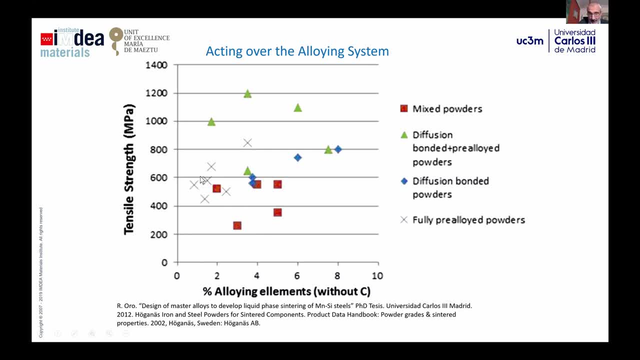 You can go to diffusion powders and pre-alloyed powders and you increase the properties, And you can go to fully pre-alloyed powders and you can get the best level of properties. So, just acting over the allogeneic system, you can change the microstructure. 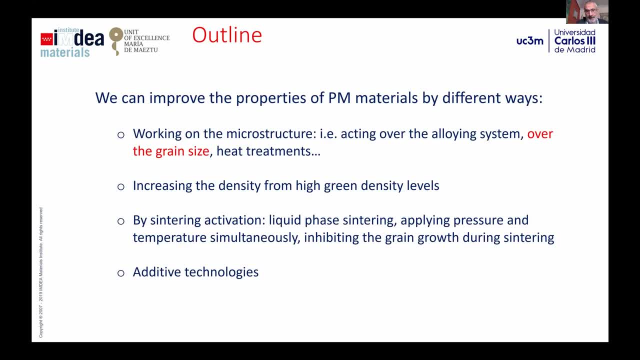 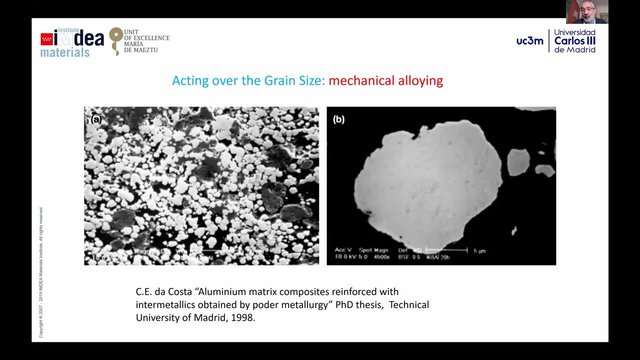 And changing the microstructure you can change the properties. Powder metallurgy is a good way to act over the grain size, And modifying the grain size you can get much better properties. One way, of course, is mechanical alloying. This is one way to produce powders in which you can get. you see, on the right, this is mechanical alloyed intermetallic obtained by mixing and milling high-energy powders from nickel and aluminium. 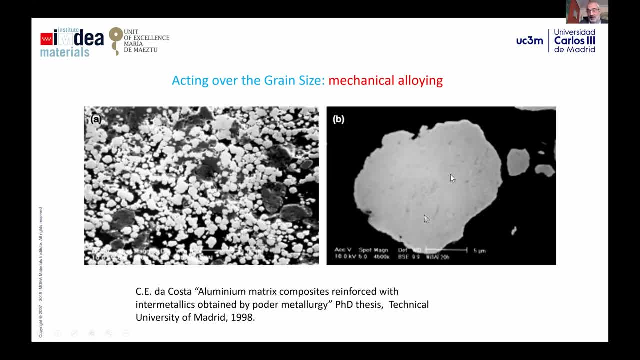 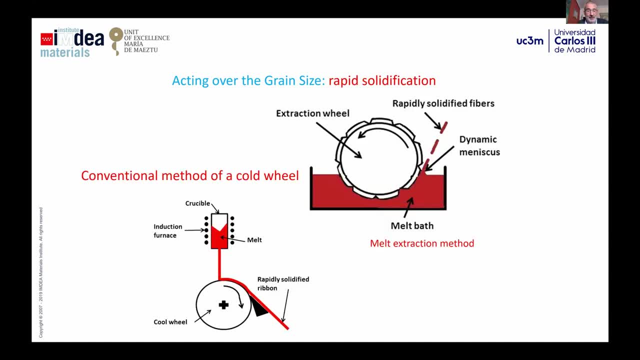 And at the end you can get a microstructure in the powder in which you have a grain size much lower than any other possibility of processing. Of course, you have also the rapid solidification methods in which you put in contact of the melt bath with the wheel, which is a very low temperature. 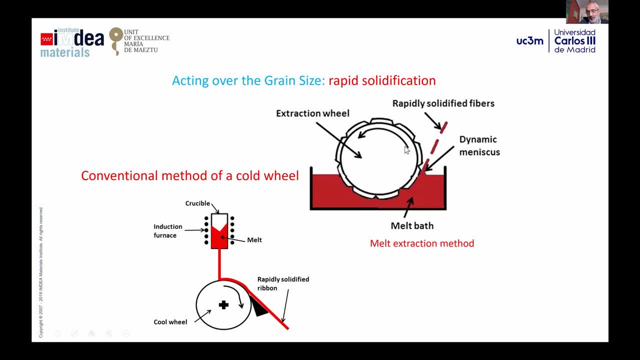 And then the solidification speed is in the order of 10,000, even higher degrees per second. In that case you are getting, in that case, fibers, Fibers that can be converted to milling in powders with a microstructure really fine, sometimes even a more good microstructure. 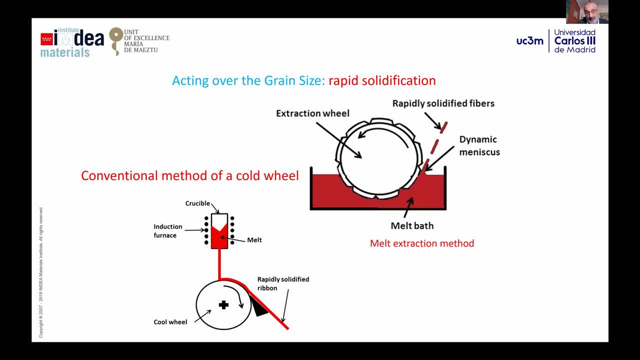 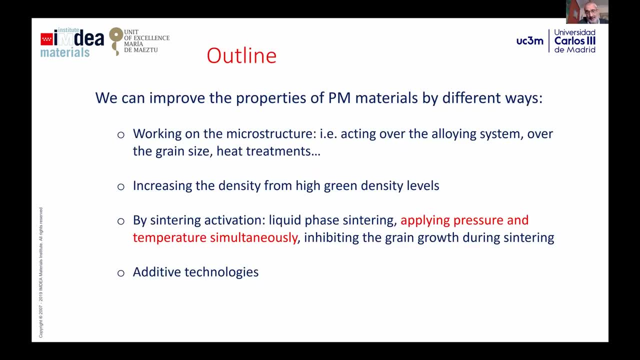 So that can. in that way you can obtain powders that can be used to develop really, really advanced materials. Let's go to the third group of methods to include the properties is by sintering activation. We have different ways to activate the sintering process. 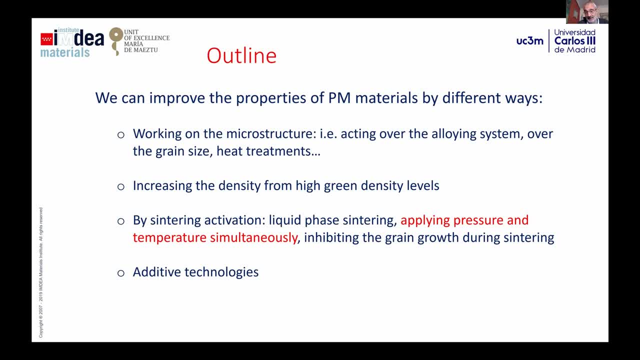 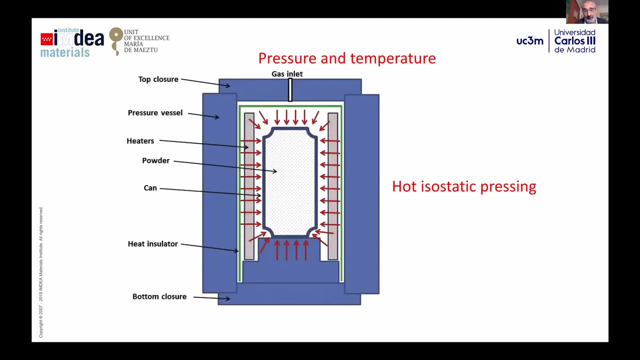 Of course, liquid phase sintering is one of those. We have different methods, But in that case we will start to talk about a couple of different ways. One is to apply pressure and temperature at the same time. This is one of the most extended methods to produce advanced materials in the last decade, in the last maybe 20, 30 years is hot isostatic pressing. 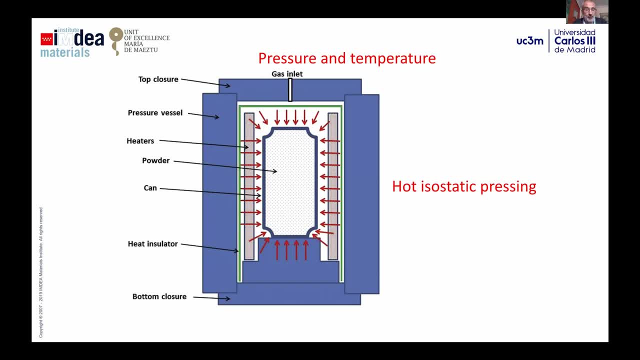 By hot isostatic pressing. you put powders inside the can and you apply the pressure to the gas in this can And you can get at the end a fully dense material with a very homogeneous material. You can control the microstructure and, of course, very good properties because you can control very well the chemistry of the powder. 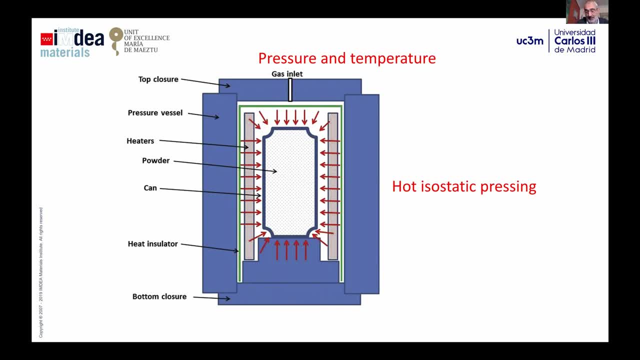 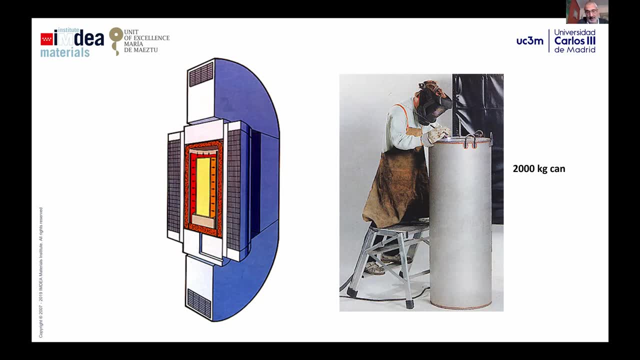 and you can control very well the microstructure of the final material. The problem of hot isostatic pressing is the price, because you need very, very expensive equipment just to perform the press and the sintering. at the same time, You have usually to can the powders inside the can and this increases a lot the price of this method. 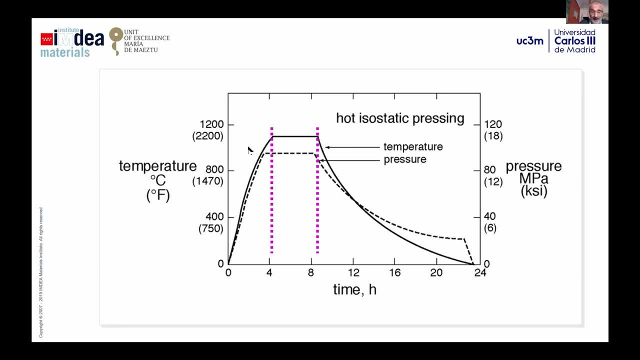 So another important thing in hot isostatic pressing is that usually you need a long period of time to reach the good properties at the end of the process. The dual time that you need to reach these properties is in the order of hours 2,, 3,, 4 hours. 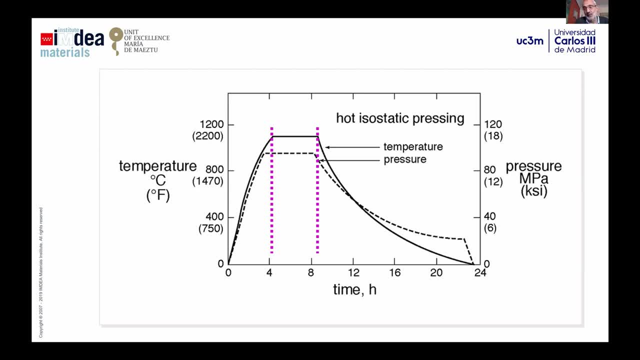 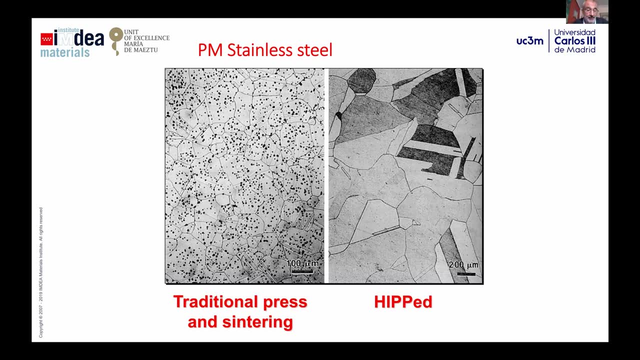 So that means it's a long process. that usually makes it quite expensive And in terms of the microstructure, one of the problems of hot isostatic pressing is that you need so long time to reach the good properties at the end of the process. 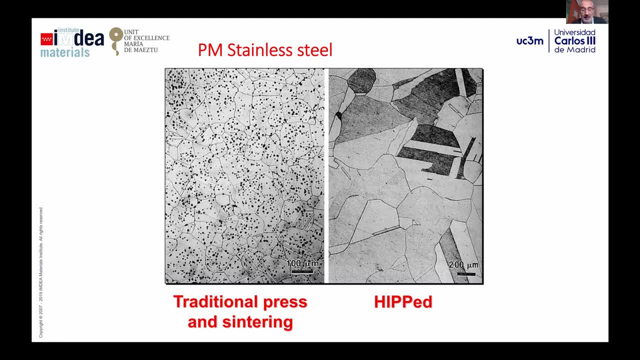 So that means it's a long process. that usually makes it quite expensive times to reach the correct microstructure. of course, if you see on the left, you have a high traditional presence in the stainless steel in which you see the microstructure, with a lot of 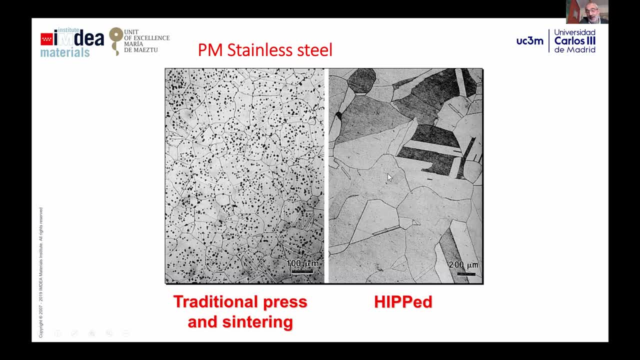 porosity. after heaping you get a fully dense material without any porosity. you cannot appreciate the porosity here, but due to the fact that you have need such a long time to reach this microstructure- usually the grain growth- more than the desire that you are deciding. 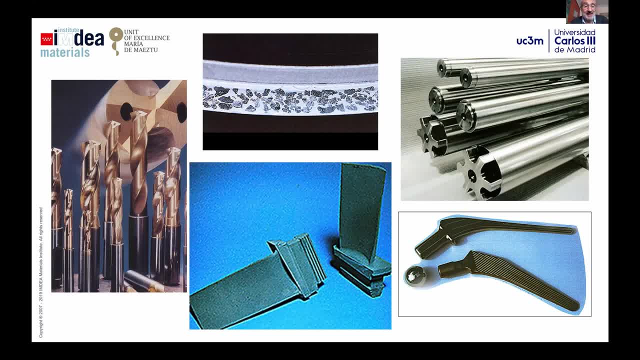 so anyway, in that case, how this person has been used for many, many years to produce, for instance, high-speed steels as you have here, this, this, this ingots of high-speed steels with the best properties that you can reach in any other possibility or alternative method. 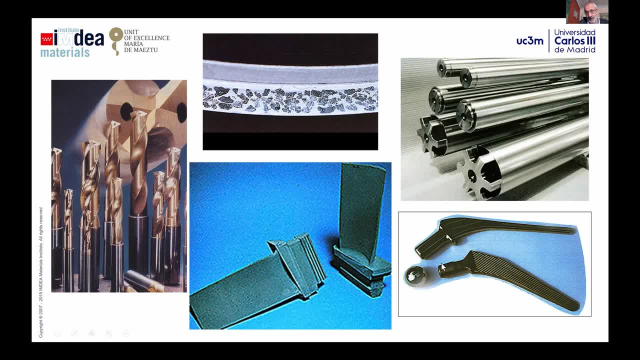 you can obtain biomaterials from different super alloys or different titanium-based alloys. you can obtain dissimilar materials, welding one base material with one, with one, composite, for instance, or blades for the for the for the airplanes, or cemented carbides for cutting applications or any. 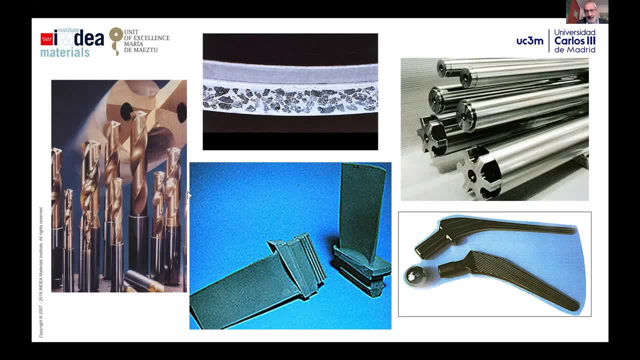 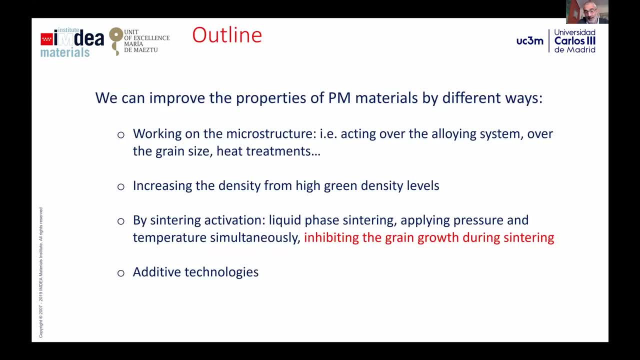 much, many other applications, is really one of the methods to obtain advanced materials in the last 20, 30 years. so we have another ways to to improve the properties in powder metallurgy. one is try to inhibing. try to inhibit the grain growth during sintering. there is one method in which you can inhibit the ring with its microwave furnace, with 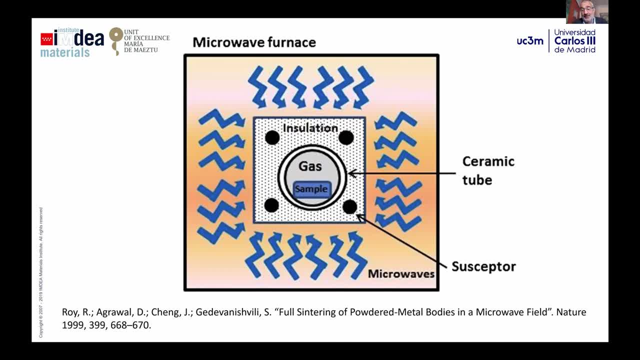 the microwave sintering. the microwave sintering was applied for ceramics before the then the 2000 year, but from 2000 year it was developed methods to to sintering in microwave furnaces even metals. uh, microwave synthesis can can reach very high. 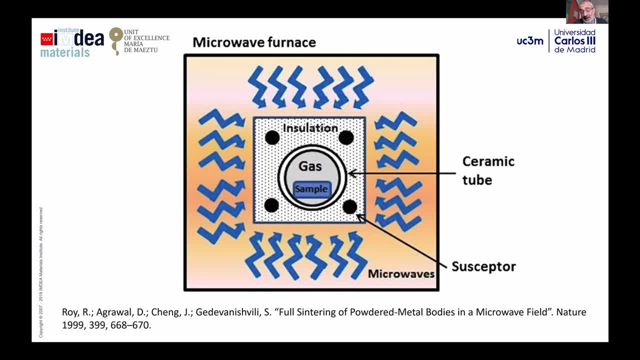 temperatures in a very short time. so that means that the dual time for the sintering is not so high and you avoid the grain growth and you can reach a good microstructure with very fine range without not so much problem with this technology but the most extended in the last times. 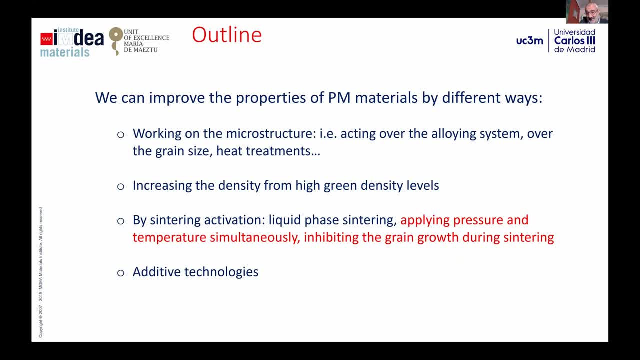 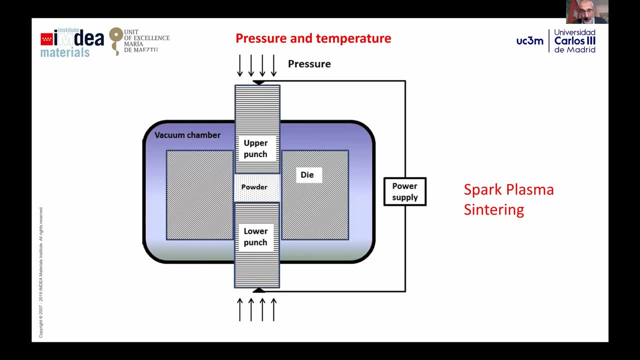 method to inhibit the grain growth and applying at the same time pressure and tempera and temperature, is the so-called fill assisted methods. in the most. the most well-known is machined name, the spare: plasma sintering. you put the powder in the dye and you apply the 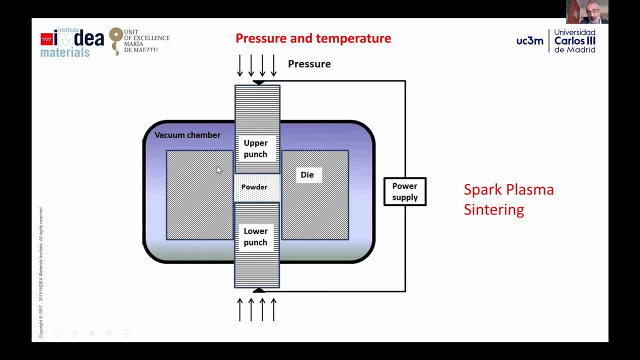 pressure with an upper and another punch. usually we we have, we have to use, in order to allow the current, the current passing to the powder, the dyes and punches of graphite, and we are applying temperatures to the uh, to applying a current through the powder and by dual effect, we are 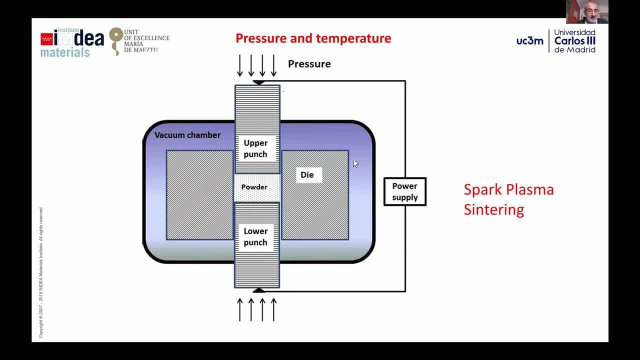 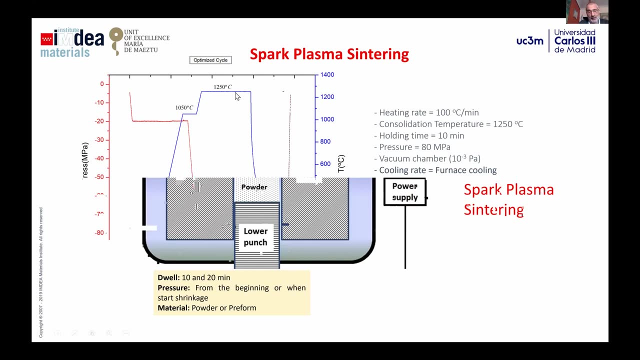 hitting the powders in a very fast way and we can reach the sintering temperatures in the pathway and we don't need so long periods to reach the full density in this material. as you can see, in this typical, typical cycle you can reach in the order of 12- 50 degrees in a very 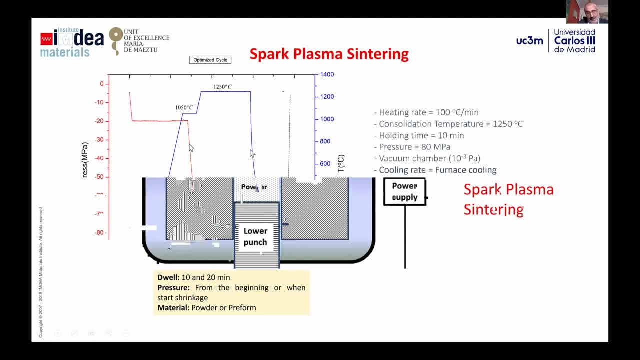 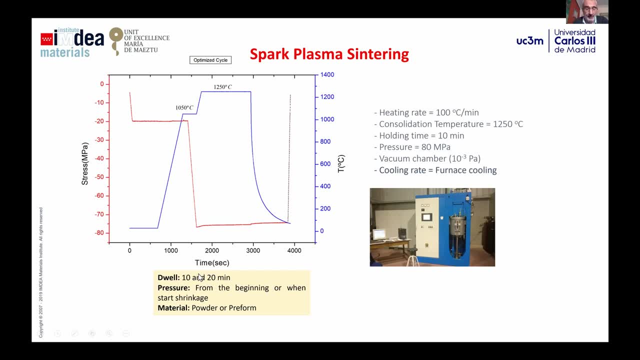 short time of time and the dwell time for reaching the the best properties in this material the people have. full density is in the order of 10, 15, 20 minutes. so if you compare with how hot is static pressing and you need more than two or three hours sometimes to reach the. 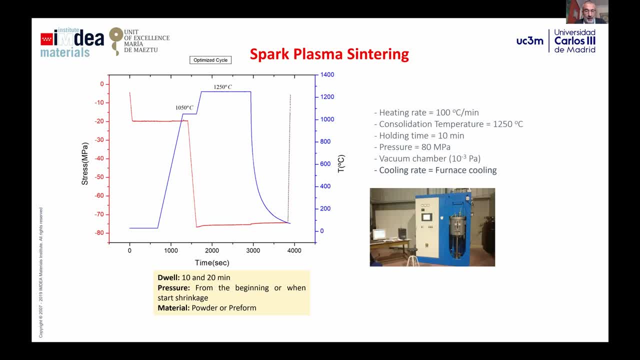 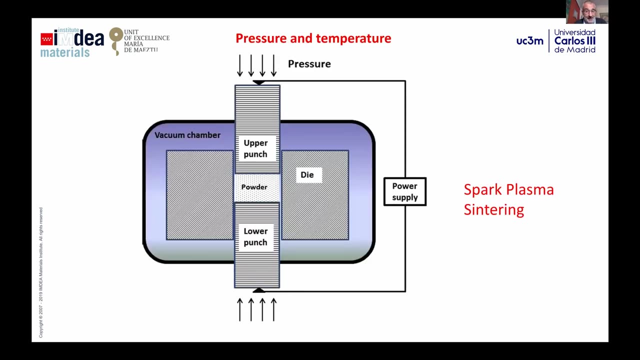 full density. at the end you are having a way to get, let's say, advanced materials but controlling much better the microstructure, controlling much better than inside with such a kind of methods. but one of the negative things of sparkless machine, the technique that usually was established, that 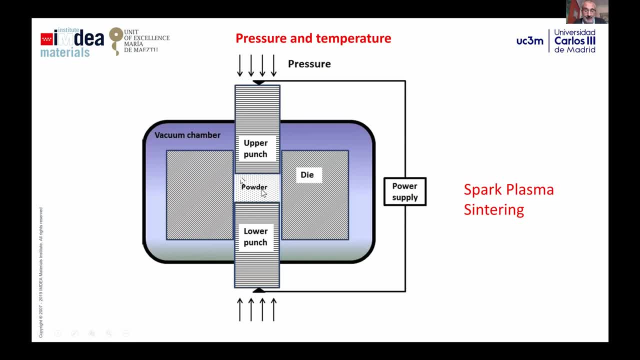 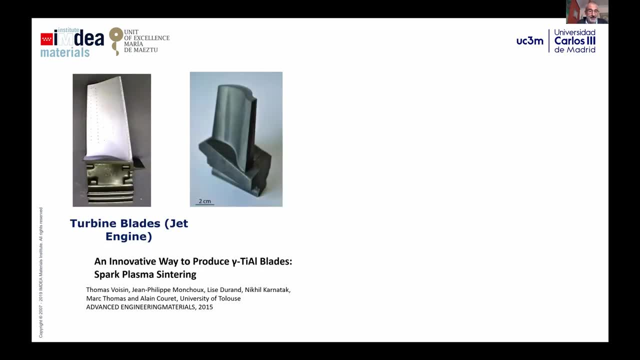 the shape is just a cylinder, it's just a blank that should be machined later in order to get the parts. but recently there is some words in which, thanks to modeling, thanks to the, the computational modeling of all the process, you can develop dice and punches that can optimize the current passing through the powder and you can get directly. 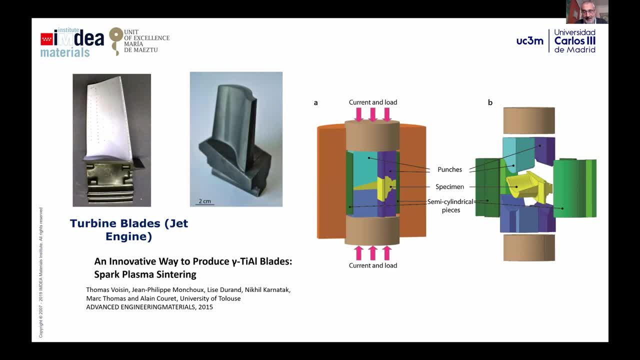 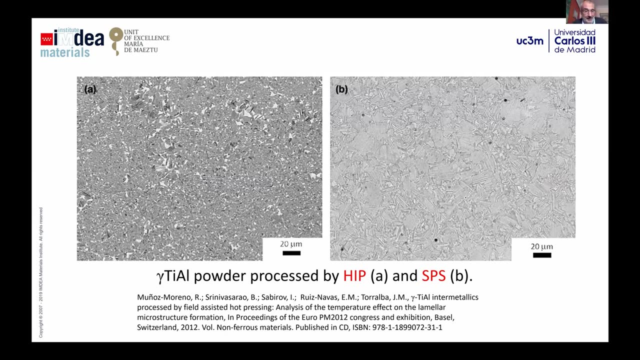 the shape of a turbine blade and you can directly obtain the final part by a spark plasma sintering. so this could reduce much the price of this kind of methodology. and just to to show some of the versatility, let's say, of the powder metallurgy, is that having the same material, exactly the same material, the same powder? 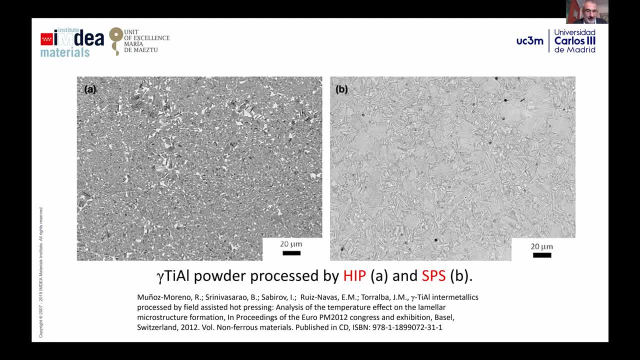 with just the same conditions, you can get completely different microstructure using different powdered metallurgy technologies. in this case, this is a work from dr muñoz on the left- you have, with one titanium aluminate powder, a completely different microstructure, a granular microstructure. the different even. 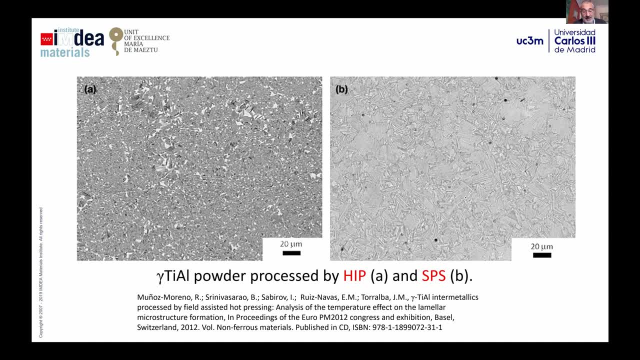 places present on the microstructure than on the right. with the spark plasma sintering which we have, we have reached the the dwell part of the processing much in a much faster way and at the end you have a better, proper microstructure for the planning application for this titanium. 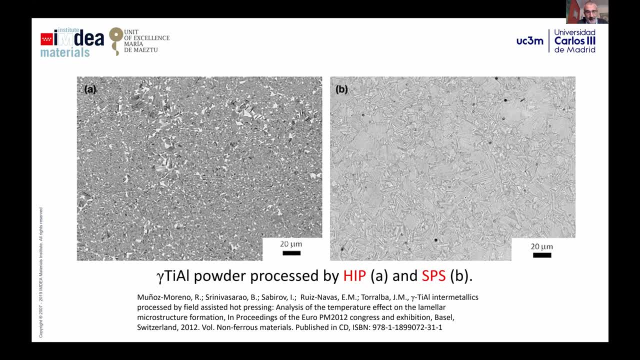 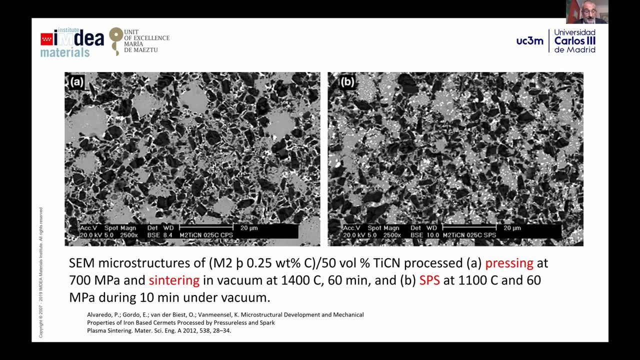 aluminate. but there is another examples in which power metallurgy has different ways to reach more or less the same material. here we have- This is produced by Pablo Alvaredo and other authors- in which you see, on the left, one material which is a composite, an iron-based composite with titanium carbonitrides, just. 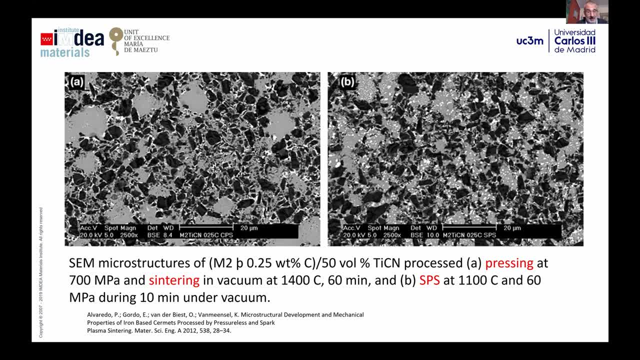 for cutting applications. You can get this microstructure on the left by pressing and sintering, but you have to reach 700 megapascal in pressing and 1,400 degrees- sorry, 1,400 degrees- in the well time of 60 minutes to reach this microstructure. 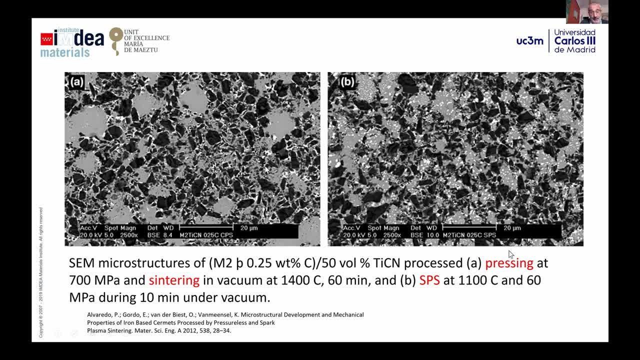 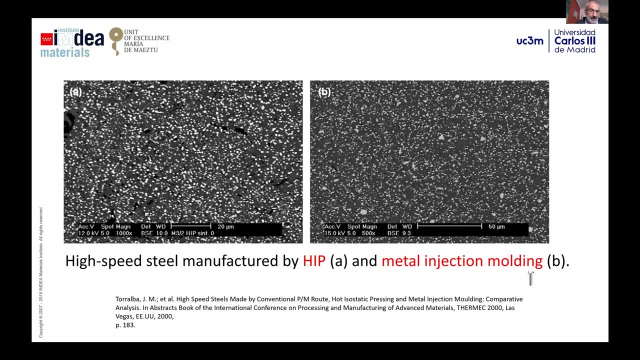 By spire plasma sintering at much lower temperature and lower pressure and just 10 minutes, you can reach a much better microstructure with more refined grain, but for the same application with much better properties. There is another example. This is one example in which you can compare. 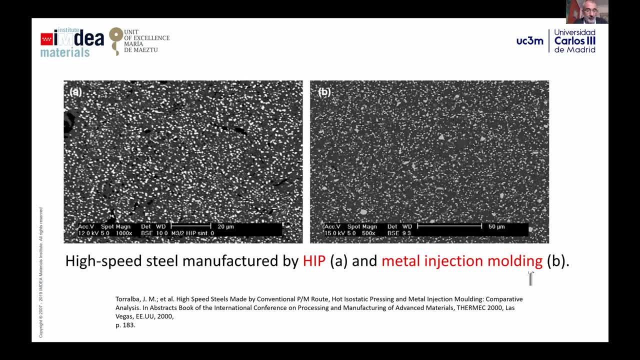 One high-speed steel on the left produced by hot isotopic pressing, and on the right metal injection molding. You can see more or less the same microstructure by different routes. That means powder metallurgy offer a lot of different possibilities to get at the end. 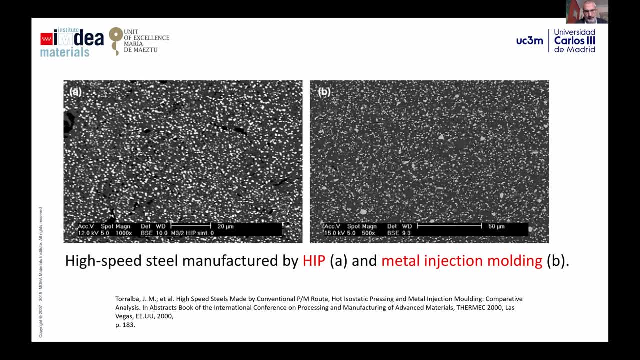 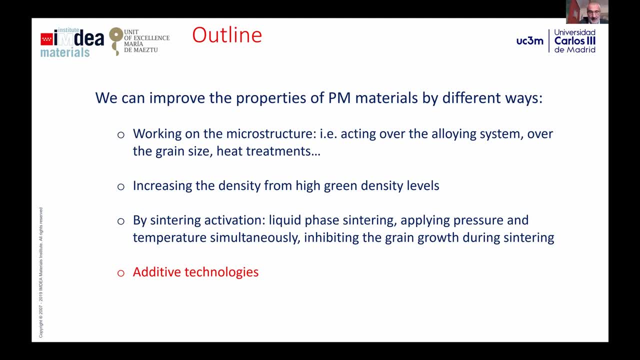 one suitable microstructure for one specific application. Let's go to the fashion of the last time, which is additive technology. With additive technologies in metals, we can reach at the end a customized material, a customized part for one specific application in a very short time. 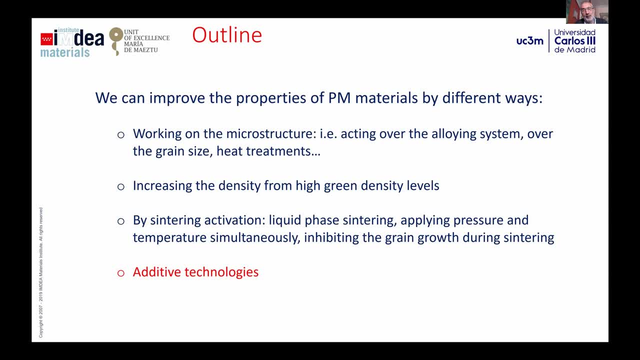 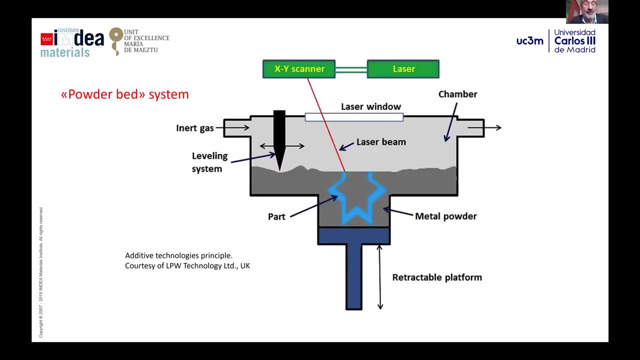 Usually we can reach good properties if we optimize the process in a good way. But even additive technologies has different possibilities, like in the other powder metallurgy technologies In IED manufacturing we have in principle three main ways to reach the final pass. 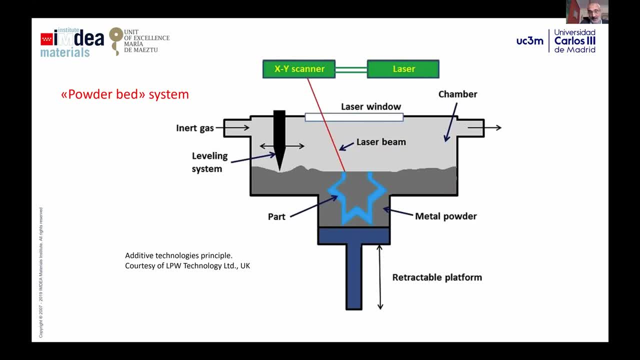 One are the so-called powder bed systems, in which we have a bed, In which we have a bed In which we put the powder, the beam, the laser beam acts on the surface and with this detector platform we can grow the part from the top to the bottom. 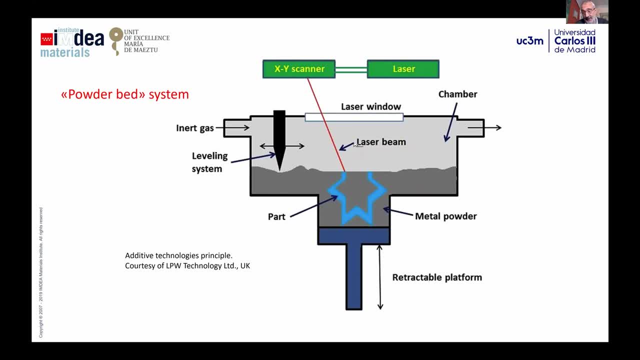 In this case, the main different thing regarding the other IED manufacturing methods is that we need for sure, fully powder with very well-controlled microstructure and well-controlled in order to assure a good melting on the upper part in which we can apply the beam of the laser beam. 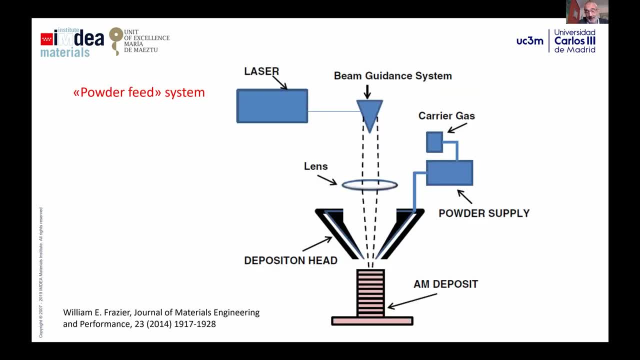 We have another alternative, which is the so-called powder feed system. The advantage of powder feed systems in this case is that we can use a mix of powders. We have different hoppers, We can feed the powders by different hoppers and we can have different kind of powders. 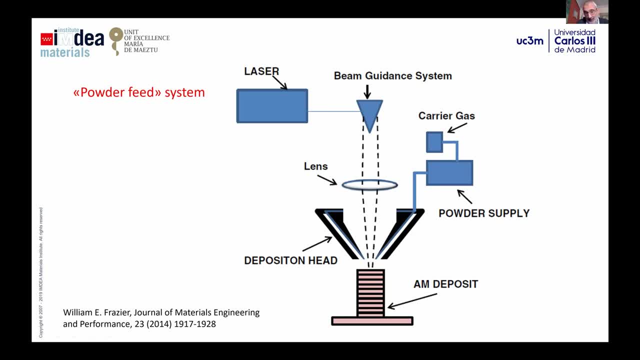 and we don't need to use a fully prealloyed powder always, Of course we can use fully prealloyed powders also. Here we have a different concept In order: how we can build the part, because here we have a bottom-up method. but at the 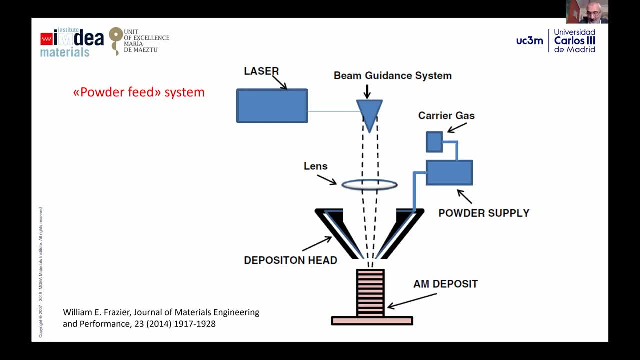 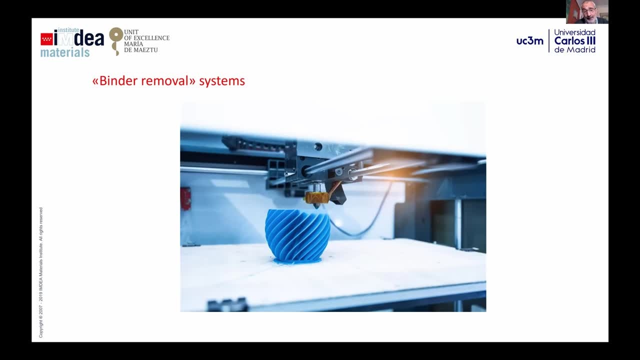 end. we have also different problems. We have a third way to obtain materials by IED manufacturing of metals, which is the so-called binder removal system. In this case, we are printing in a similar way that we print the parts in 3D printing. 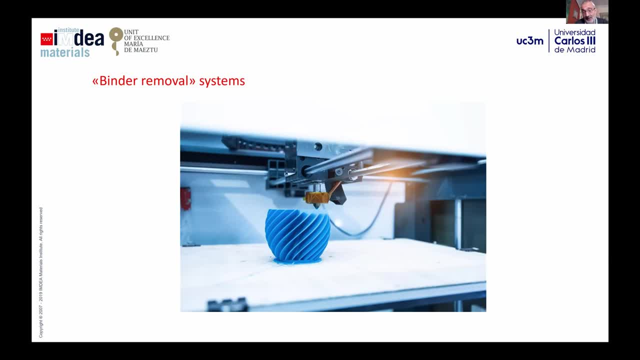 for polymers, but in this case we need a feedstock. We need a mix of polymer and metals In order to have a good printing method. In this case, once we have the printed part, we need to remove the binder. 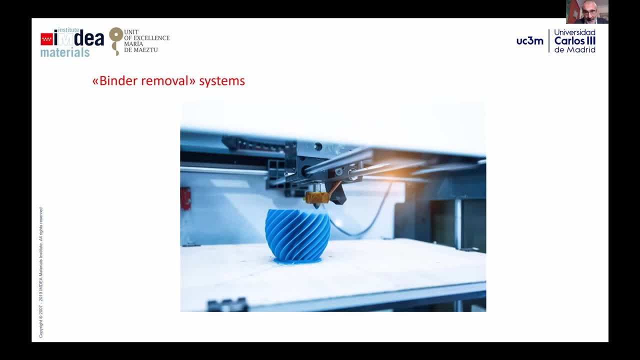 Sometimes the amount of the binder is not so high, like for instance in the HP method. HP method, in which we have a very small amount of binder, but there is other methods in which the amount of binder is much higher. Once we have removed the binder, we have to move the part to a sintering furnace and 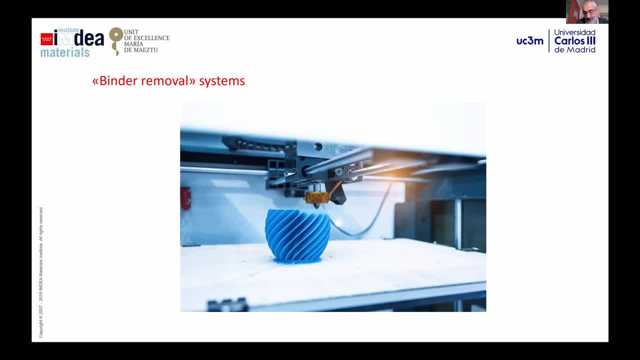 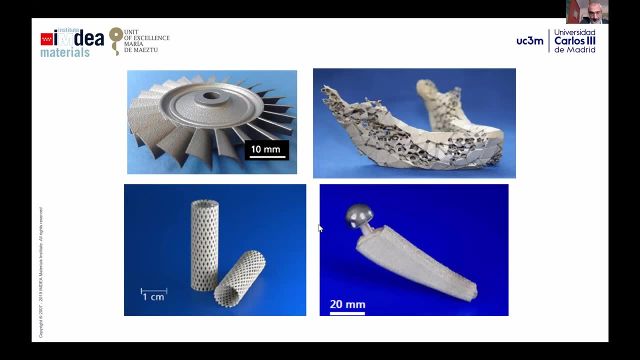 then to reach the final product, Thank you. So the final product is, after the sintering process, the conventional sintering process. So by IED manufacturing, as you can imagine, you have the possibility to tailor the porosity. 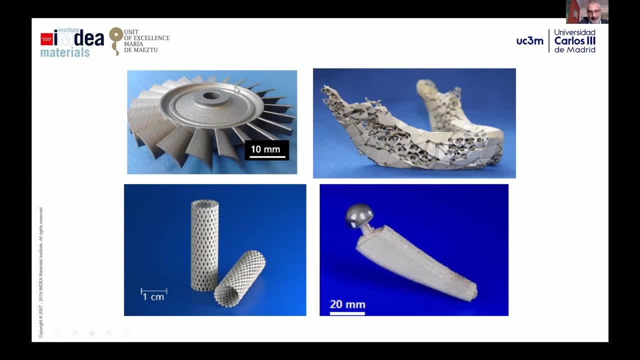 in different shapes and in different kinds of materials. You can get parts for various mass materials for aerospace or for airplanes And of course it has a lot of applications in biomaterials for implants and for a lot of applications in biomaterials. 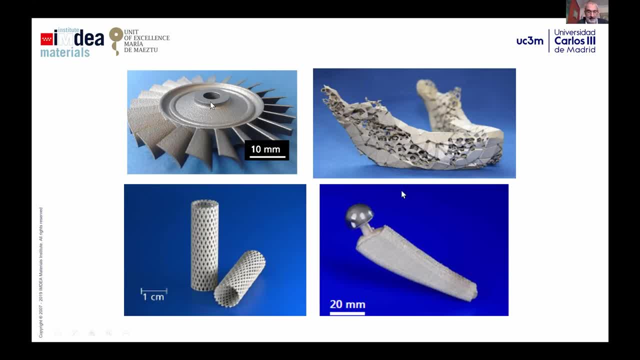 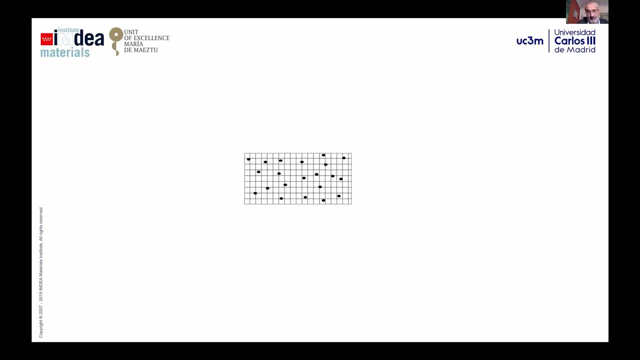 in biomaterials. So this is really a revolution because you can customize the part and you can customize the method to produce the final part with very specific properties for some specific application in a very short time. This is one of the advantages. 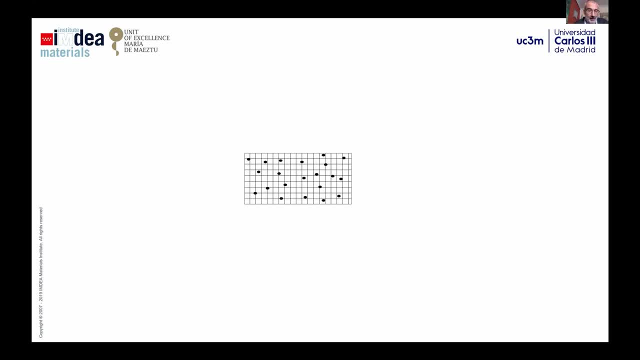 So in powder metallurgy most of the people know the powder metallurgy in which you have porous material that you have here. But just modifying the alloying system you can go to different microstructure And even you can control the grain size by methods. 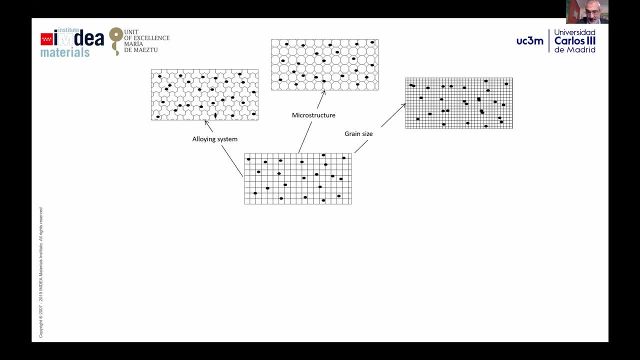 like we have seen, like mechanical alloying or rapid solidification techniques, But also with powder metallurgy you can reach through high grain density Or by cinder activation you can reach near full density materials Here. I can draw here some porosity. 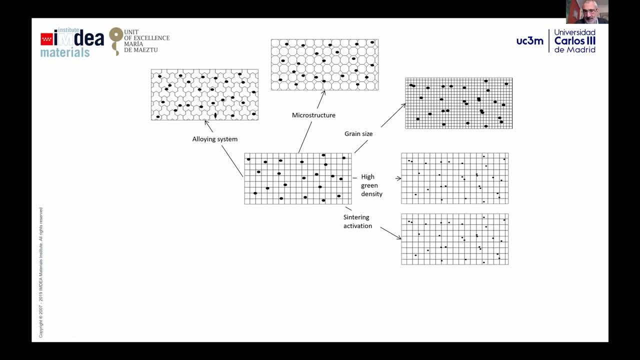 But this porosity is really, really small. even sometimes it's difficult to be detected by a lot of characterization methods. Of course you can apply pressure and temperature. You can inhibit the grain growth with methods as I mentioned, like microwave sintering or spark plasma. 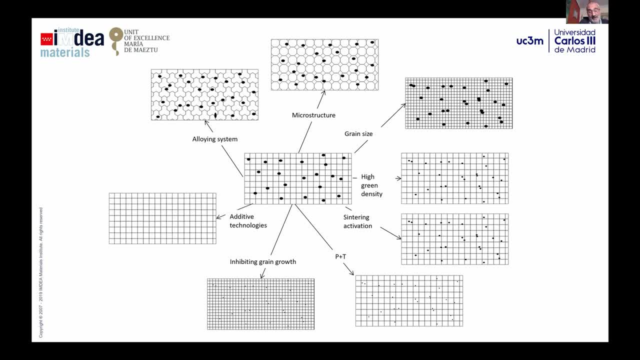 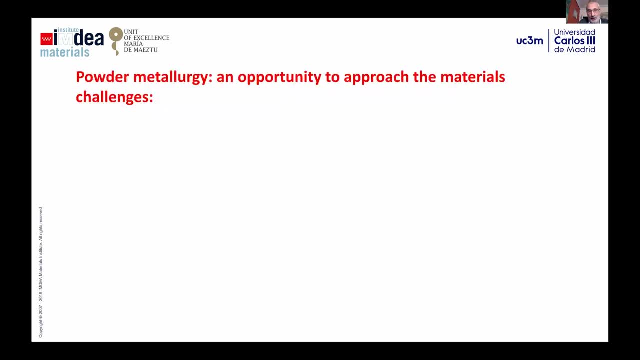 sintering, And today we have a last way to obtain full-dense material with additive technology. So we can say that powder metallurgy can offer a lot of opportunities to approach the so-called material challenge, as is the name, but also the process. 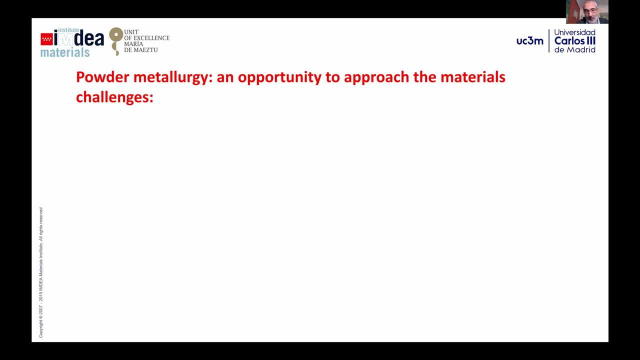 Thank you, That's the name of this lecture. So I will focus on two different material challenges in the industry and in the new technologies. One is the high-temperature challenge. The high-temperature challenge is really important in some industries, But maybe the main battle war that we 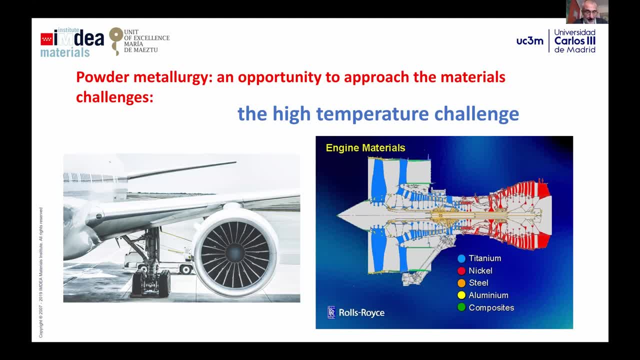 have in the high-temperature challenge is in the airplanes. in the airplanes, especially in the engines. In the engines you can find many kinds of materials: titanium-based materials, nickels, steels, even aluminum aluminides and even ceramic composites. 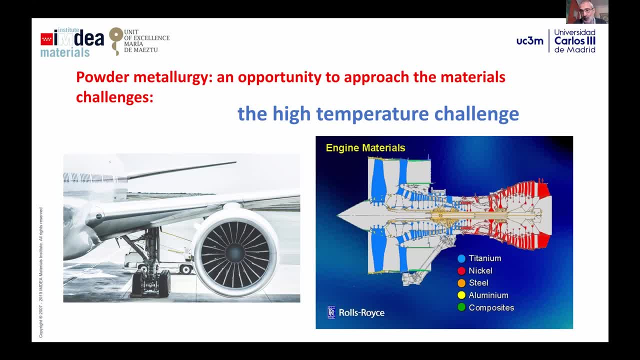 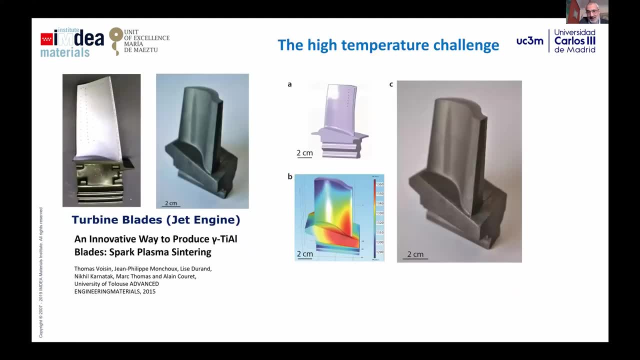 in which the battle to reach a space, a place to work, is really, really hard. In that case powder metallurgy offer a lot of possibilities. I have mentioned before the spark plasma sintering, which through this technology, you can reach really advanced materials. 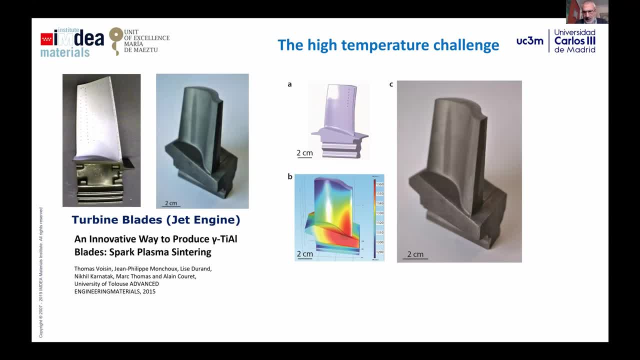 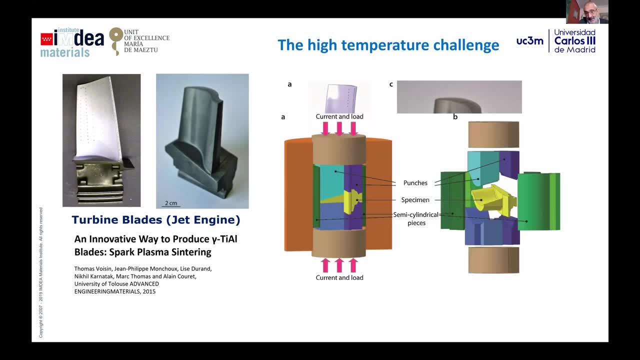 with a very well-controlled microstructure with highly suitable to compete with any other competitive alternative processing technology, Thanks, in that case, to the combination of the technology with the modeling, in that case to design the dyes and the punches, But also the powder metallurgy offer a lot of challenge. 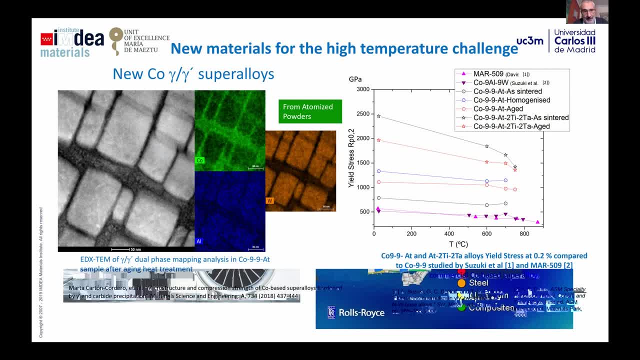 a lot of opportunities in the development of new materials, because the way in which we produce the alloys allows to us to do things that are not possible to do in alternative technologies. In this case we have. this is the microstructure with the new cobalt gamma-gamma-prime superalloy. 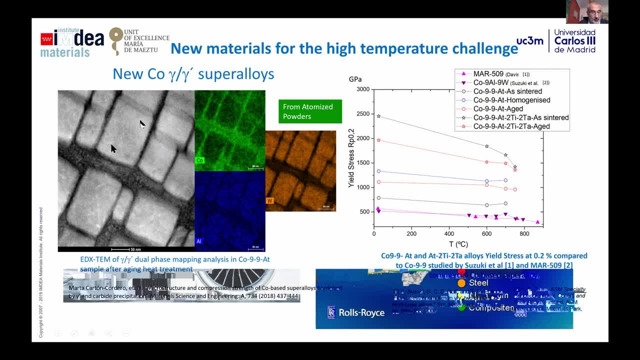 in which we can reproduce the conventional superalloys, nickel-based superalloys, microstructures, And in this case, through powder metallurgy, we can reach much better properties than using alternative technology. This new superalloy was developed in 2004, 2005.. 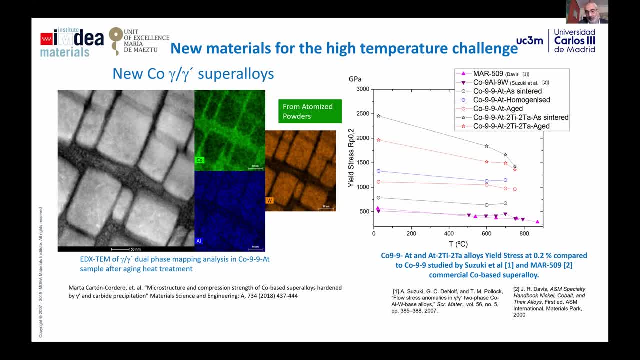 In the last year, we have been working through powder metallurgy in order to improve this alloy. In this case, here we have the results we have obtained for this alloy in conventional cobalt-based casting alloys, but also using casting to this specific superalloy. 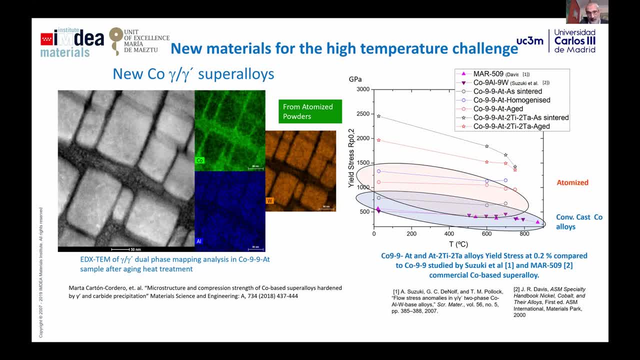 But by powder metallurgy, using fully atomized powder, we can improve much better the stress as a function of the temperature And even by addition of different alloying elements. by mixing the powders and by mechanical alloying through the atomized powder, we can also 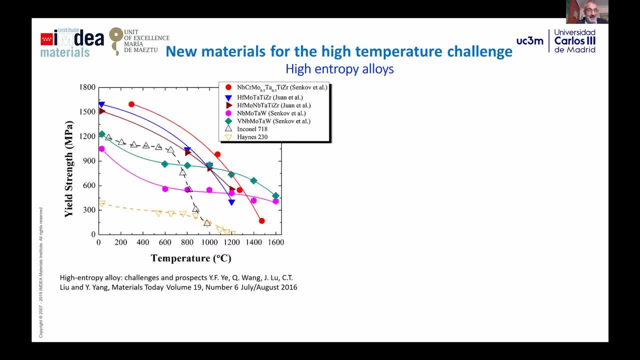 reach much better properties. But in the last year we have been working with a lot of different materials And in this case we are finding a lot of new materials. One of these new materials has been developed in the last, let's say, 10 years. 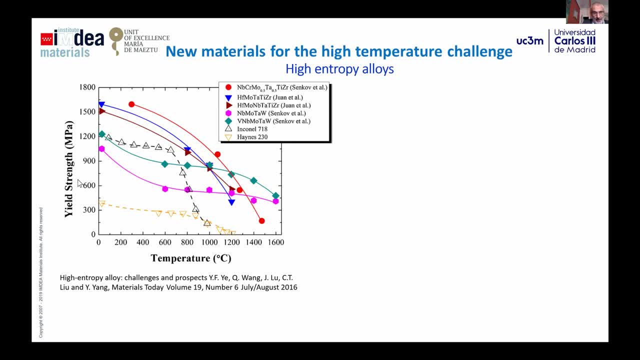 It's high entropy alloys. In high entropy alloys you see the correlation in between strength and the temperature. This is a material that can compete much with the wood advantages with conventional inconel or other nickel-based superalloys which we have here. the behavior: 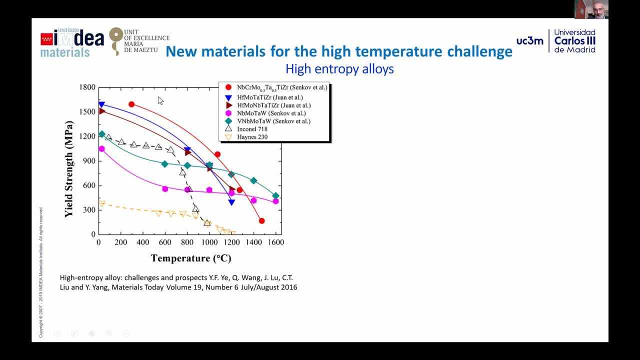 against the temperature. Here we have the, The new, let's say high entropy alloys. So we have moving the course in this way, in which we have much better behavior with the temperature. But this high entropy alloys, of course, can be produced by ingot casting, but also by powder metallurgy. 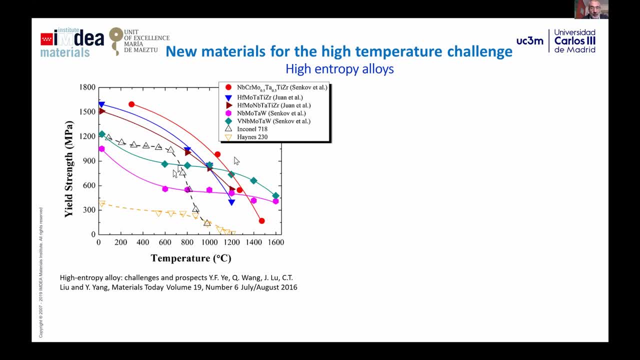 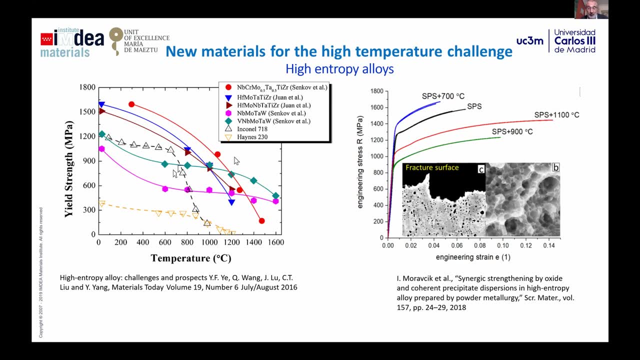 But by powder metallurgy we can do things that are not possible to do with conventional ingot casting, For instance the development of the so-called ODS- high entropy alloys- in which we can disperse. We can disperse oxide, We can disperse nitrides in the high entropy alloy. 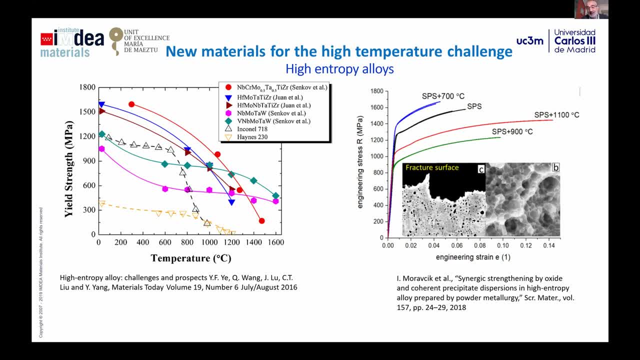 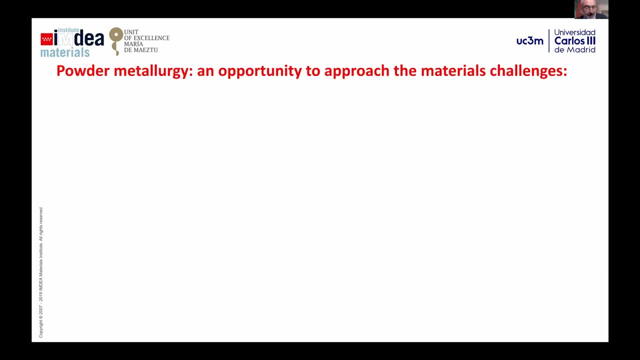 through spark, plasma sintering and other powder metallurgy technologies, We can reach this exceptional, let's say, in comparison with conventional ingot metallurgy, high entropy alloys. So we have another field. This is the field of the high temperature challenge. 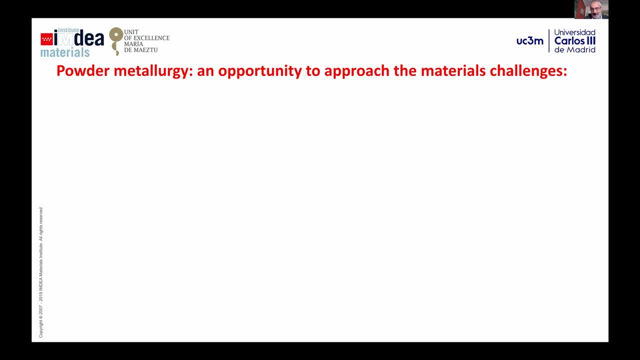 But we have another field in which we have a real important challenge for material science, which is the functional material challenge. And specifically there is a lot of application in which we can functionalize very well the properties of the final material thanks to the powder metallurgy. 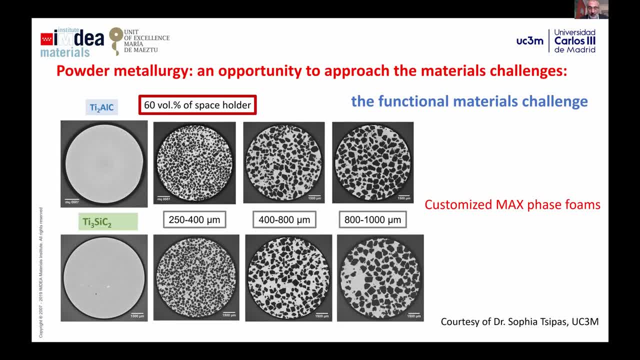 technologies. This is one example- This is courtesy of Dr Sofia Tsipas from Carlsberg University- in which you can see: here we can combine a new material with a new technology. The new material is the max phase- max phases- which is a new kind of materials. 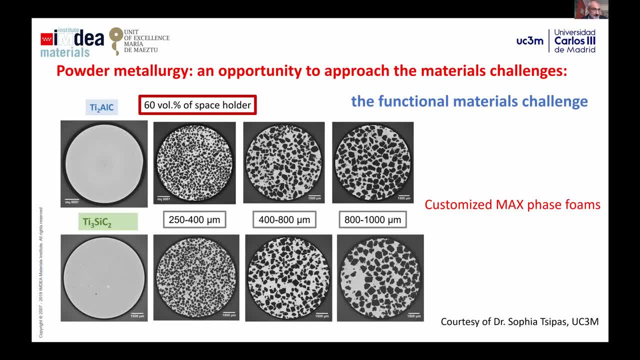 in which we can combine three kinds of alloying elements, such as titanium, aluminum and carbon, or titanium, aluminum, silicon and carbon, in which we can customize the porosity thanks to the space holder technology in powder metallurgy. 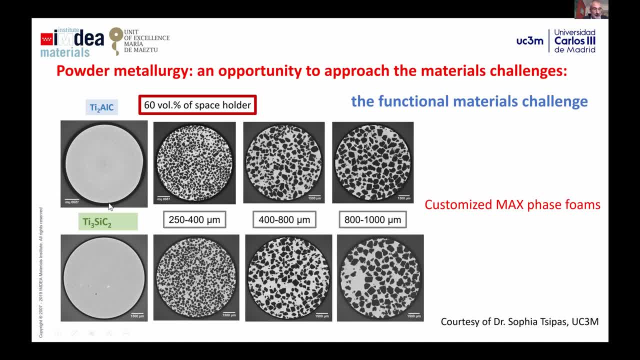 On the left you can see a fully dense material that can be obtained, But you can customize the porosity for different kind of application, in which we can obtain, at the end, porosity with a very well-controlled size, in this case between 800 and 1 millimeter. 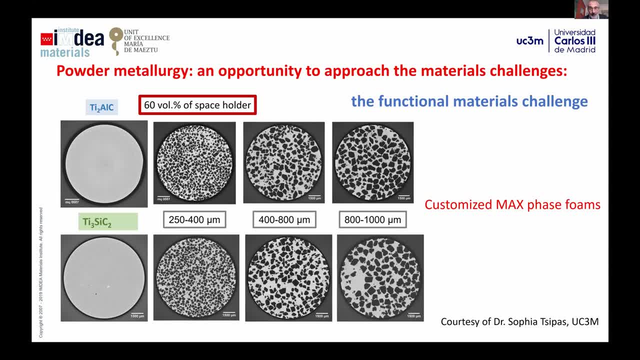 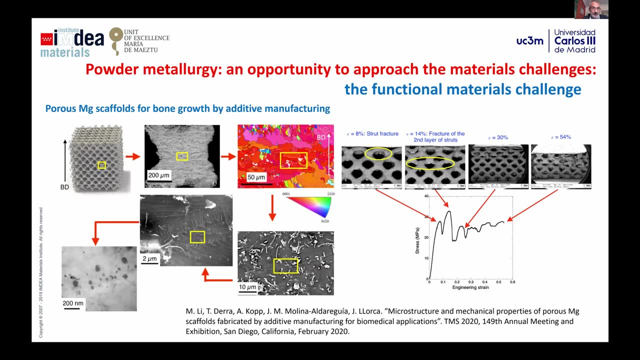 So that means that through powder metallurgy you can really develop material, But for some specific application, just working, acting on the alloying, let's say the alloys that you are working with, but also with the technology. Here we have another example. 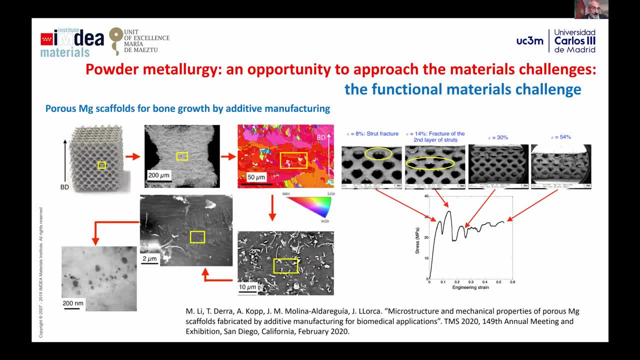 In this case, it's the development of porous magnesium scaffolds for bone growth, in this case by additive manufacturing. Additive manufacturing is a fantastic technology that you can customize a lot of things. You can customize the level of porosity, You can customize, let's say, the size of the strut. 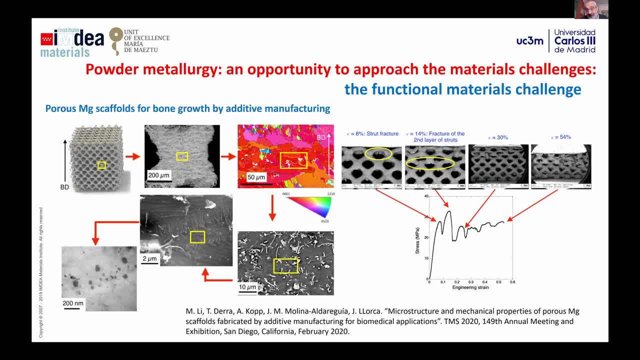 in that case, In this case, in the case of the scaffold, And even you can design how could be the strength and elongation of each strut that you have in this specific part. So for bio-application, you have a completely new world. 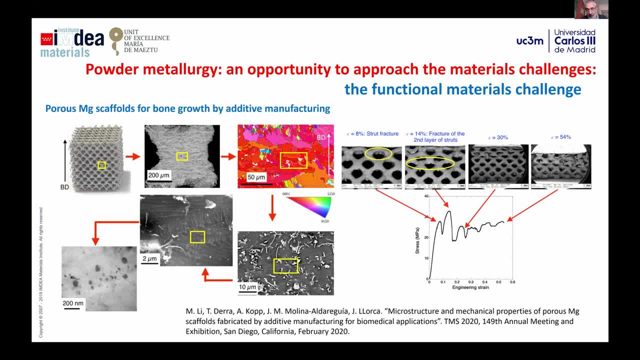 thanks to the combination of the new materials with new technologies, in this case based on powder metallurgy, In this case additive manufacturing. And let's go to the last example, which is a very, in my opinion, amazing, amazing. 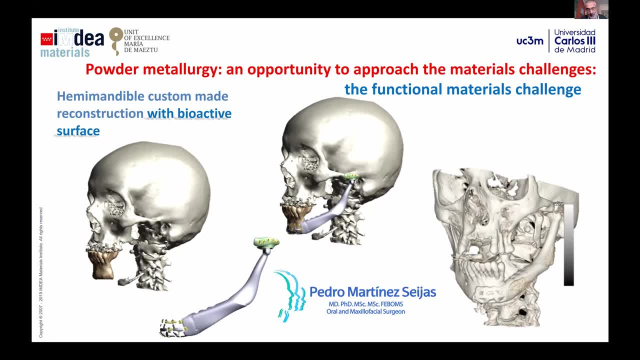 And this is thanks to the courtesy of Dr Pedro Martinez-Seijas, oral and maxillofacial surgeon, This doctor, he can develop. This is made in Spain, fully made in Spain. He can develop a handy-mandy, custom-made reconstruction. 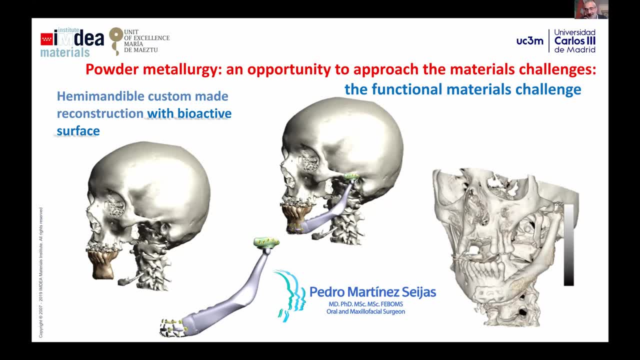 with a bioactive surface especially developed for one specific person, And you can construct This. you can design the new mandible by CAD systems And then you can reproduce exactly what you need on the patient by additive manufacturing, in this case, metallic additive manufacturing. 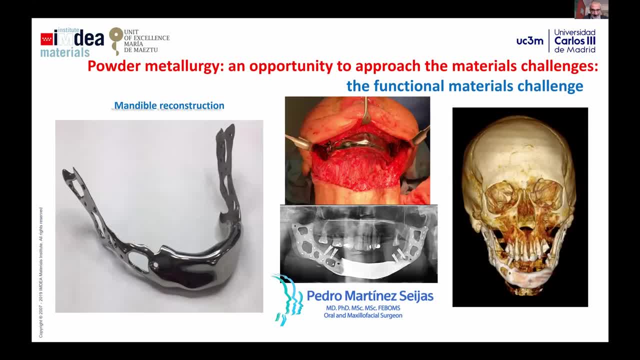 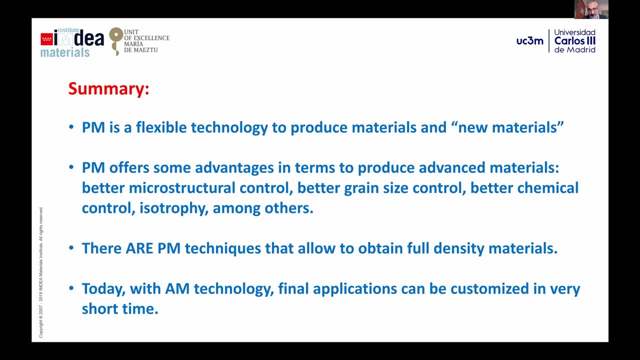 This is one example, But here we have another amazing example in which you can reconstruct a fully mandible reconstruction by additive manufacturing of metals. So we have seen that powder metallurgy is a real flexible technology That can produce materials and new materials. 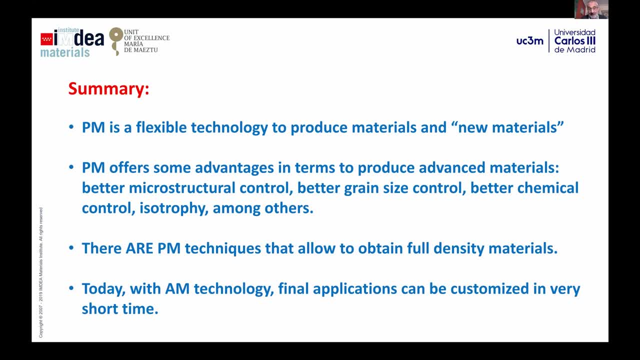 advantages in terms of produce these new materials, because we can have, of course, new technologies developed especially for these new materials. But you can control the microstructure much better than any other alternative production method. You can have much better grain site control, of course. 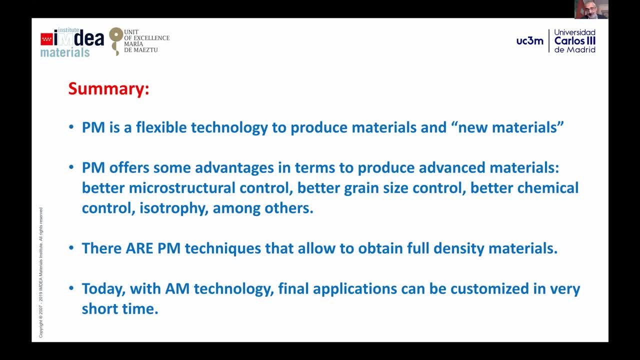 much better chemical control, isotropy, among other advantages. There are a lot of PM techniques that allow this full material And today with the additive manufacturing technologies, you can get a lot of final application that can be really customized in a very short time. 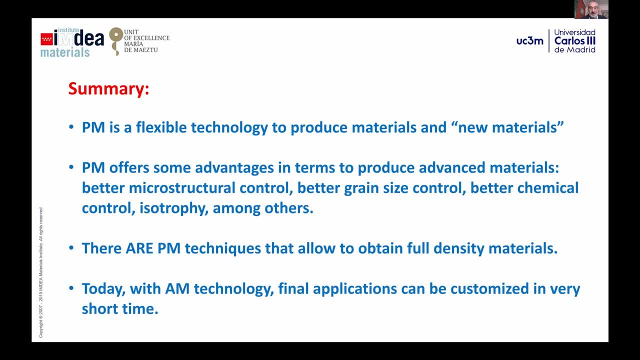 You can have in a very short time a mandible. You can have in a very short time a heap. You can have in a very short time one specific part to replace one fail that you can have in one advanced process that you are running in one specific application. 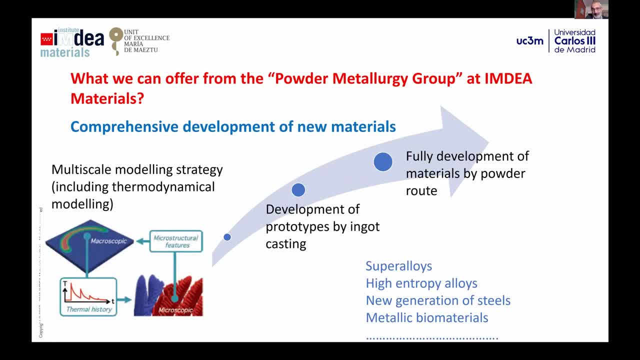 So what we can offer from the powder metallurgy group in their materials. One interesting thing that we can offer is that we can really comprehensively develop new materials from the beginning till the final part. We can really develop the material from the beginning. 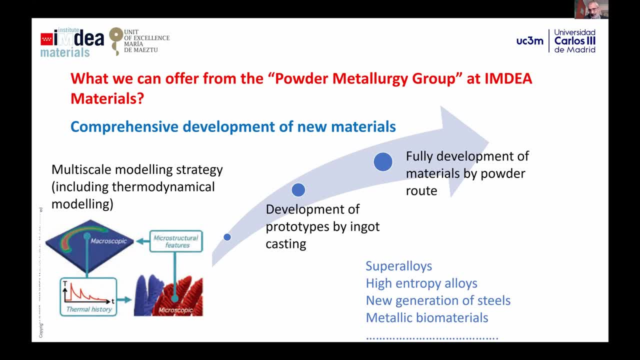 because we can combine one, let's say, important skill that we have in the institute with a multi-scale modeling strategy, from the atom to the final part, including the thermodynamic modeling of the materials, Of course. once you have developed the, you have designed the material. you can develop prototypes. 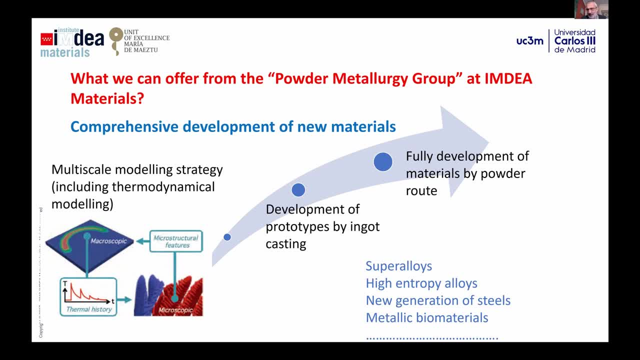 in that case. And then you can test this microstructure and you can reproduce the microstructure by different ways, And then you can fully develop the materials by powder route. And we are talking materials, We are talking different kinds of materials. 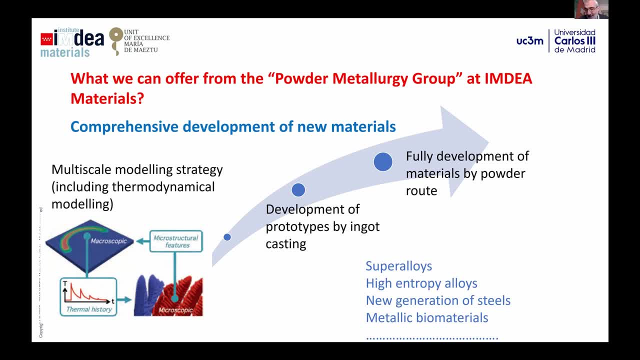 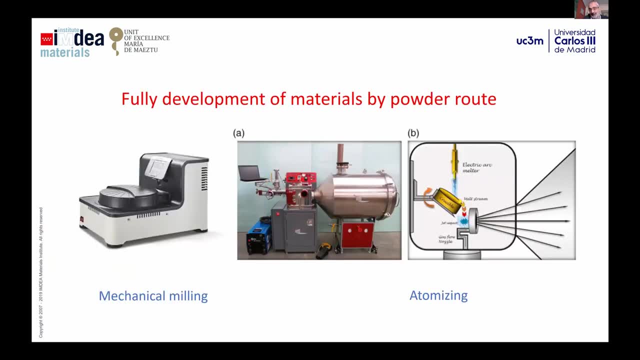 Of course, alloys, high entropy alloys, new generation of steels, biomaterials and so on. And once you have designed the material, you can develop the powder by different routes, by mechanical alloying or atomizing. And of course, then, once you have the powder, you can develop. 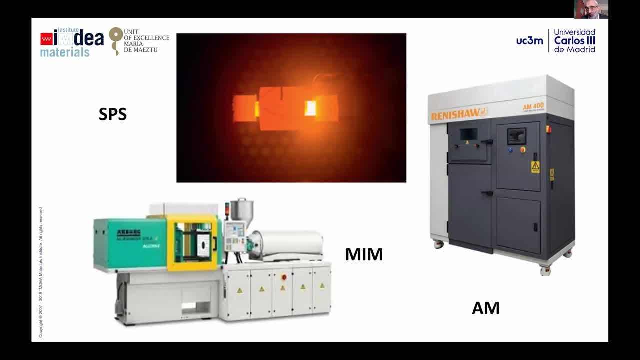 You can develop the part, You can develop the approach, the bulk material, by techniques like by fill-assisted hot pressing or metal injection, molding or, of course, additive manufacturing. But another, let's say, strong point of the institute is the multi-scale characterization. 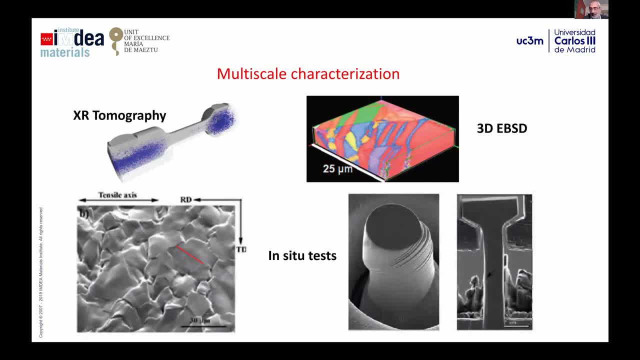 In all the process, from the beginning, from the ingot casting model to the final part, produced by one specific technique, by powder metallurgy technique. you can test in all the steps different problems that you can have in the development. You can control the microstructures. 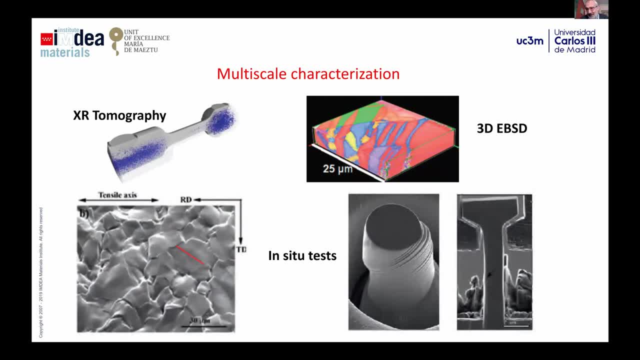 by X-ray tomography And you can develop in situ test to test very small parts or very small part of the microstructure, or even to know, to have a good knowledge of some phases that you can detect before by ABDS techniques in the field microscope. 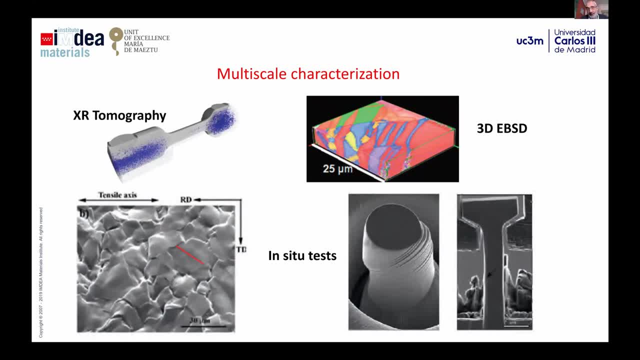 So at the end, you can combine a lot of techniques of characterization, a lot of techniques of multi-scale modeling order to develop the materials and, of course, the technologies to produce the real bulk part in the process. So I think this is all. 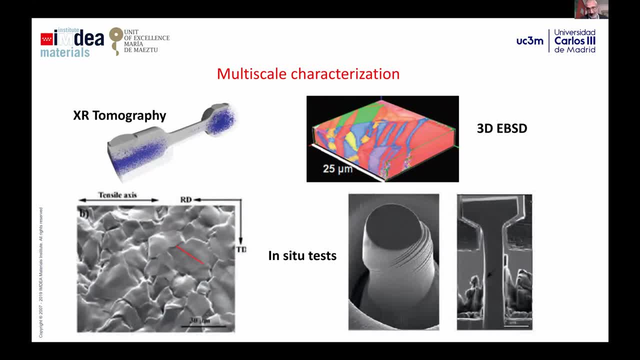 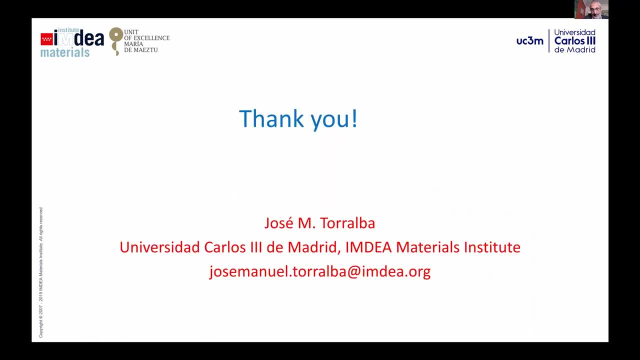 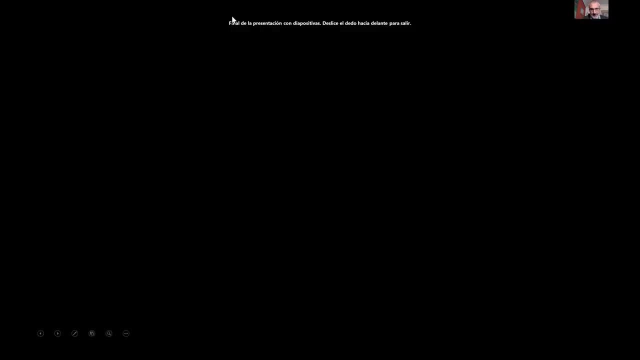 So now I think I have fulfilled the time requirements that Miguel Angel told me about 40 minutes, 40,, 45 minutes, And now I completely open and thank you to your questions. Well, thank you very much, José Manuel. Thank you very much for the presentation. 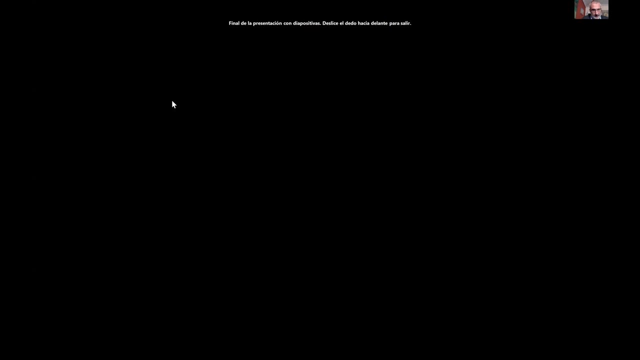 And this clear overview and you gave a very nice and open talk about the different possibilities of powder metallurgy and opening new possibilities of these different technologies and the processing and post-processing techniques associated to this methodology. So well, this is now time, for now we have like 10, 15 minutes. 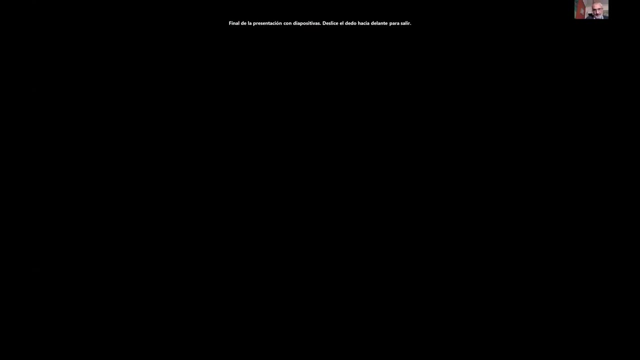 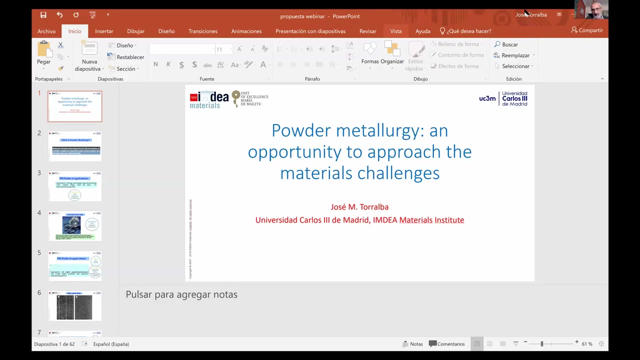 10, 15 minutes for questions. So anyone that would like to ask something to Professor Torralba, please write the question through the chat so I can read it, or Professor Torralba can read it directly, But meanwhile the people or anyone, 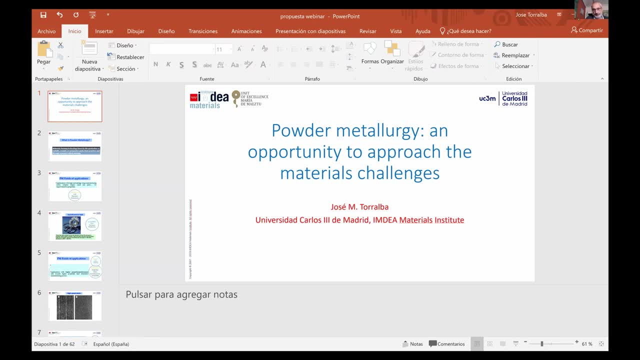 is actually writing any of the questions. I would like to make the first question. So you were talking about the high entropy alloys, So I know that this is, I mean, relatively quite new, but I would like to ask you: how implemented is this in industry nowadays? 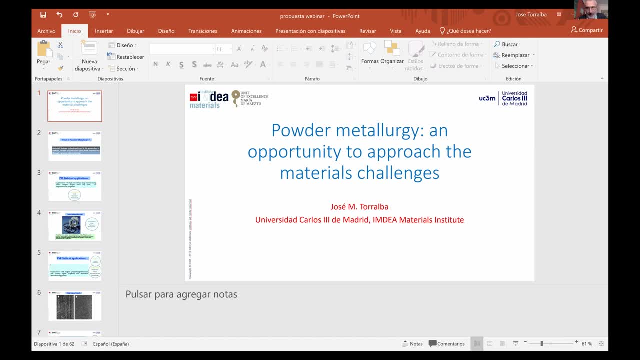 Now in industry it's completely a new field. There are some industry that I am I know that they are just thinking about to test this kind of materials. But today we are still a little bit far from the industry. because high entropy alloys needs not only technology, it needs a lot of physical metallurgy, it needs a lot of knowledge to the development of these materials. 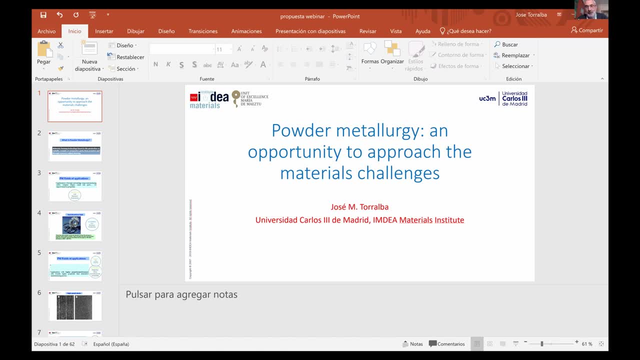 But they are really promising materials because when you are in the limit, when you are in the breakthrough of the application, sometimes you need to improve 10, 15, 20 degrees more in terms of high temperature, in terms of some specific behavior in some specific fields. 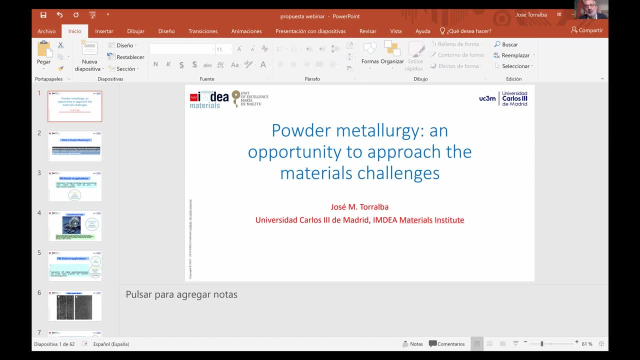 And in that case you have to go to these new materials to break through, to change the things in this such a specific application, And we are working very hard on that And we are trying to compare some high entropy alloys with conventional superalloys and with conventional intermetallics. 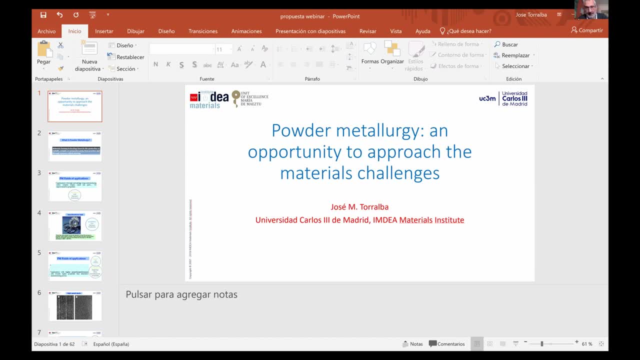 In the field of high temperature applications, And I think that these are really promising materials in the future. Okay, And what about the cost? Do you have any? Yeah, cost is in some way a little bit higher, must be a little bit higher because you are using much more amount of specific alloying elements. 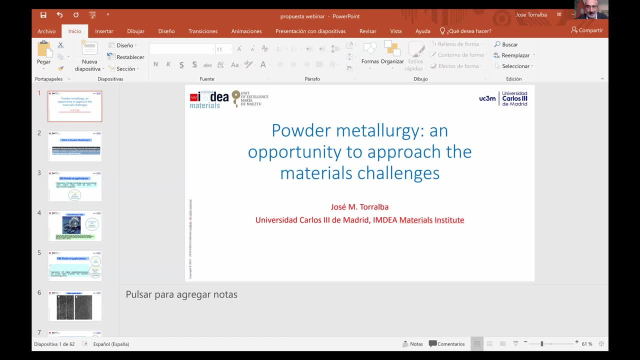 But you have to think that when you are fighting in this breakthrough, in this part of the limit of the technology, sometimes, Sometimes, cost is not the most important thing. Okay, So there is another question here. Well, the first general question that I read is about the presentation. 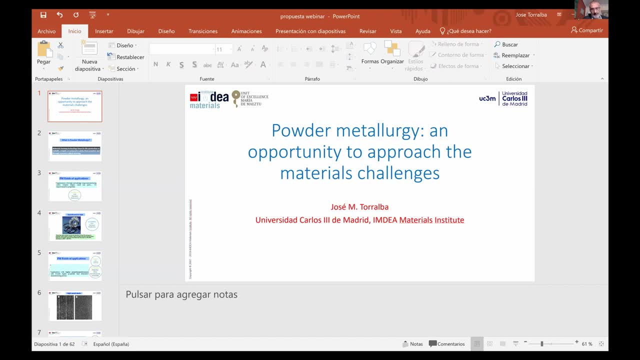 Well, the full seminar is going to be published in our website, And so everyone is going to have access to these slides and the presentation, And also, well, actually, you can go through the whole webinar If you want. any time. it will be in our web page. 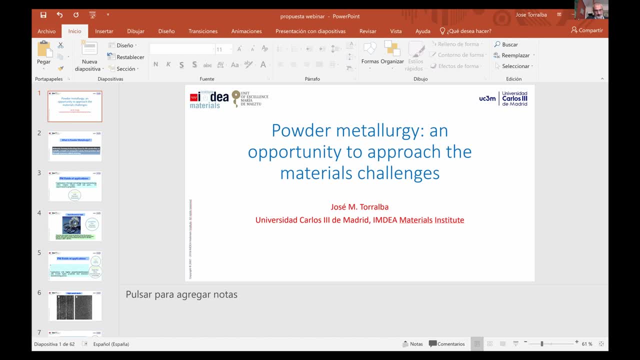 And then there's another question here, Jose Manuel, I think: are the high entropy alloys processable using additive manufacturing? Is there any particular element that has a main role in these alloys? Yes, there is. In fact, I am working in one review paper on high entropy alloys and additive manufacturing and I hope to publish it in a very short time. 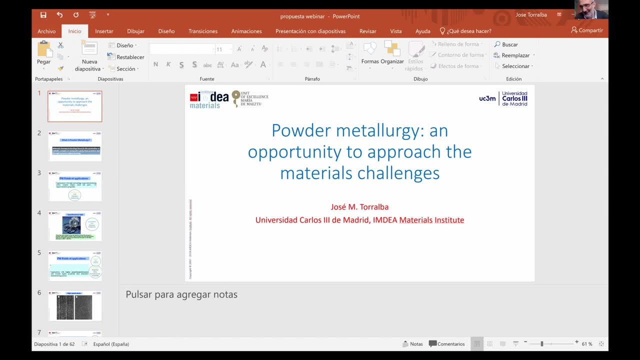 I hope so. Let's see This quarantine. I have some time to reflect on these materials. High entropy alloys: there is in the last two, three years, there are in the order of 50, 60 papers regarding high entropy alloys and additive manufacturing. 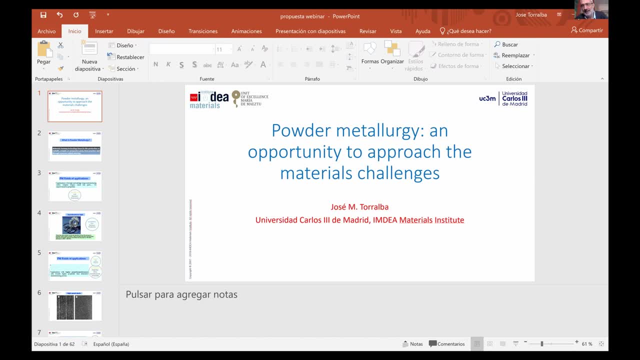 Of course, using BinderJet methods, which is maybe the more vision way to produce high entropy alloys. I think this could be a very interesting area, because by BinderJet you will use, at the end, sintering in a very similar way that. 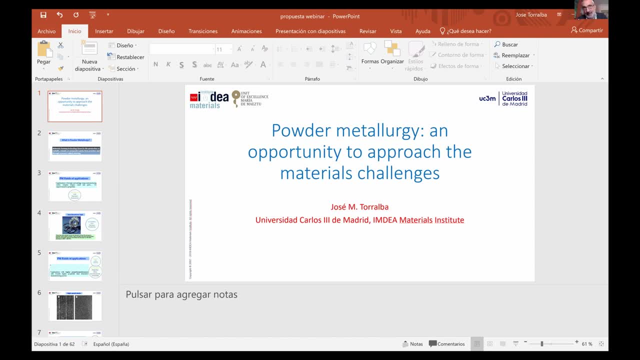 other alternatives, But by selective laser melting or even direct metal deposition. there are many, many people working on that. There are two different approaches. When you are going to select the laser methods, you need fully prealloyed powders, which is not easy in high entropy alloys to find it. 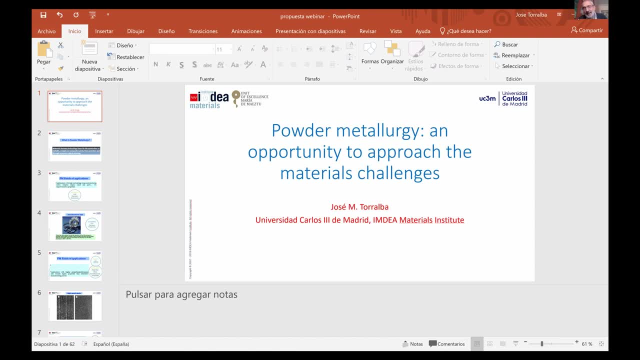 But in direct metal deposition you can mix the powders by elemental mixing. So that means that you have a lot of opportunities to design High entropy alloys, And there is in additive manufacturing. most of the people are using the so-called Cantor alloy. 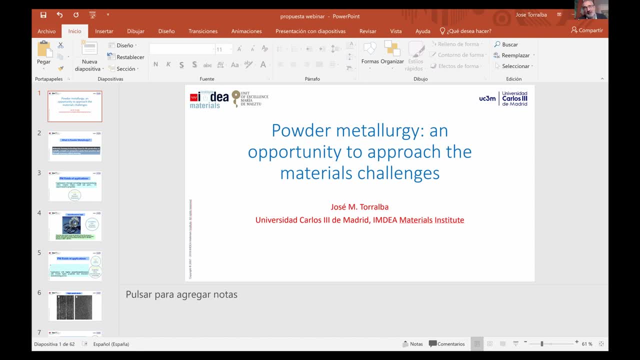 If you are in this field, you will know what is Cantor. The Cantor alloy is. Cantor was the first person to develop one of the high entropy alloys. It's iron, cobalt, manganese, nickel, chromium-based alloy. 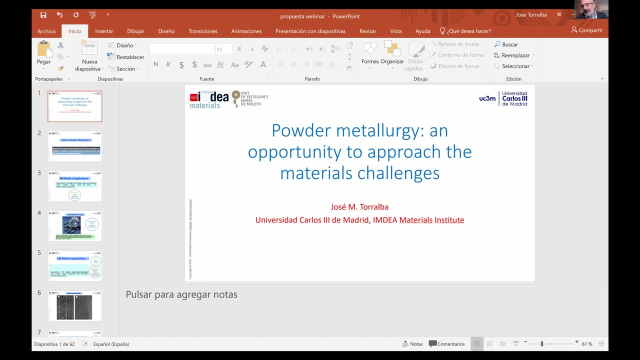 And in that case there is one element which is playing a really interesting role, which is aluminum. Aluminum in the Cantor alloy used to be replacing the manganese or even other of the other five elements, And with the aluminum you can tailor a lot, the microstructure. 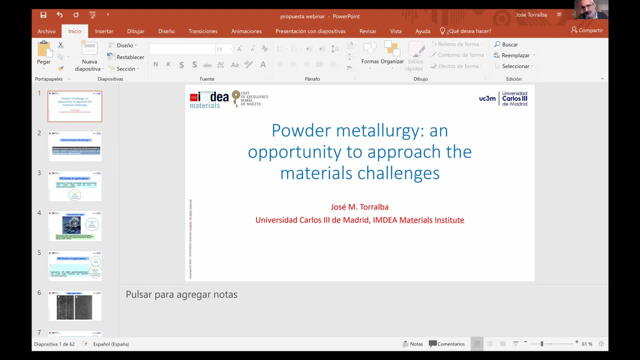 Because usually the Cantor alloy is an FCC alloy, It's a completely fully FCC phase center cubic alloy. But aluminum introduces the possibility to have a mix in the microstructure in between BCC and FCC And that play. That could play a very nice role in order to have good heat treatments, in order to improve some specific properties, especially for high temperature. 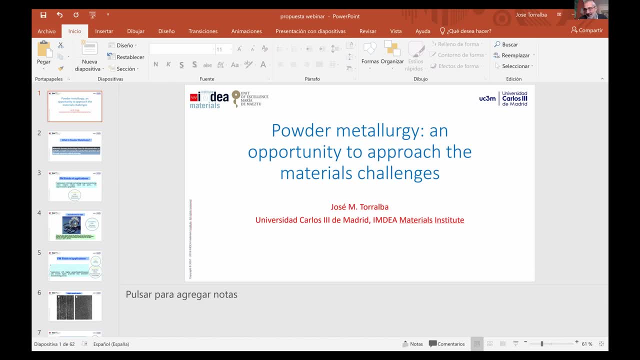 So there is an interesting field in these two emerging technologies: By one side, additive manufacturing and on the other side, the high entropy alloys as material. Excellent, Thank you, José Manuel. And another question here is: Do you Uh? 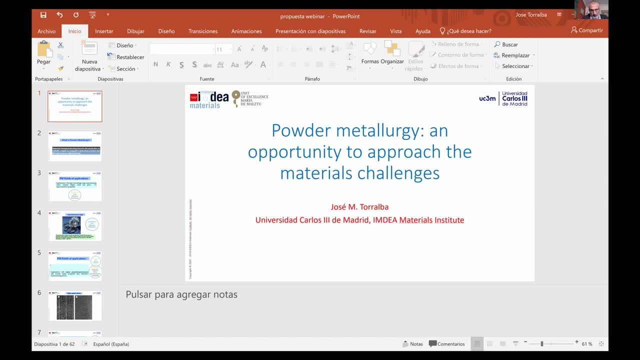 Do you think microwave sintering and SPS fast sintering techs can be commercialized in the future? Or do you think the oven companies already worked for large furnaces but they failed. In the case of microwave sintering, I think there is now so many companies dealing for that or betting for that. 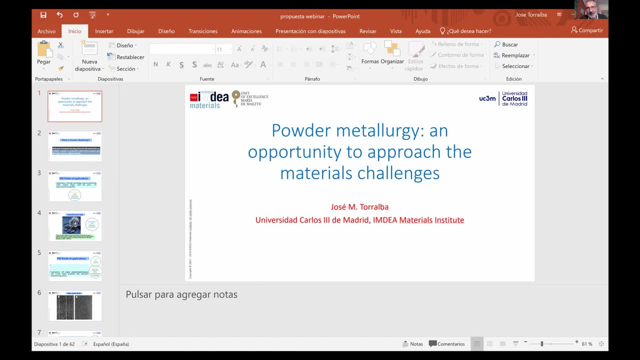 So, but I think in the future, when you have a way to reach good properties and good materials at the end, at the end, there will be somewhat who would try to do it at in this level. There is some sort of applications, but there is more. 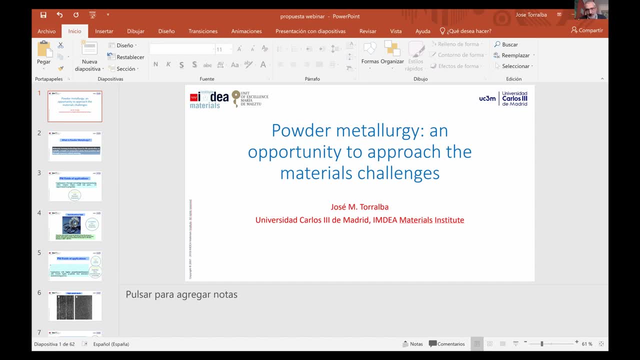 a small application and people, let's say a specific application, but it's part of much of iniciating. I think this is a real situation. they will mold or surge in the industry. In fact, there are some other space industry that they are working a lot with. this把 goes must. 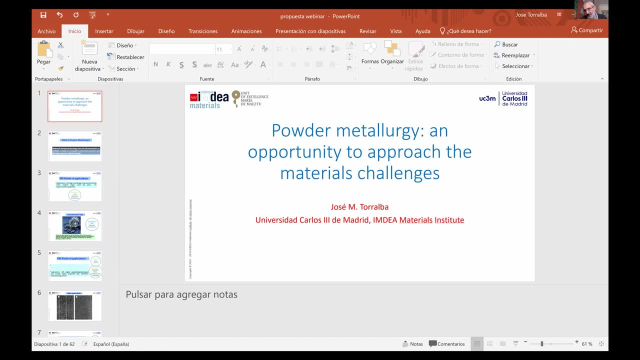 Sending a process. So in the case of№ and З saying I think we arrived at the before snakes, that just tell you exactly that. Do you think belleza sins gonna give us some more investment Because at the end, at the end there will be someone who would try to do it at industry levels? 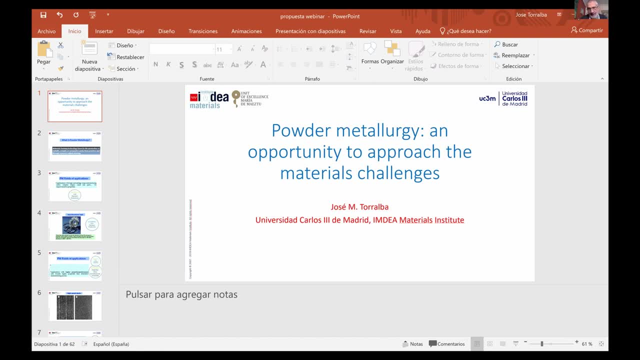 It is some sometimes, but there is more. we are a little bit far from the industry, But as far as plasma scintillating we are much more near in the industry because there are some companies which are now working and trying to develop things by spartoplasma scintillating. 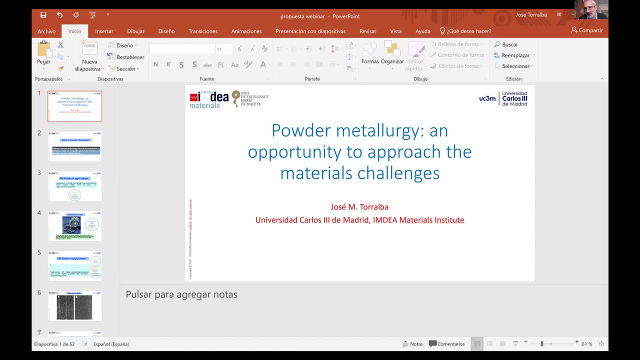 Spartoplasma scintillating in fact is like, at the beginning, hot isototic pressing. At the beginning, hot isototic pressing, the problem was the size. It was not possible to produce near-nest-shaped parts by hot isototic pressing. 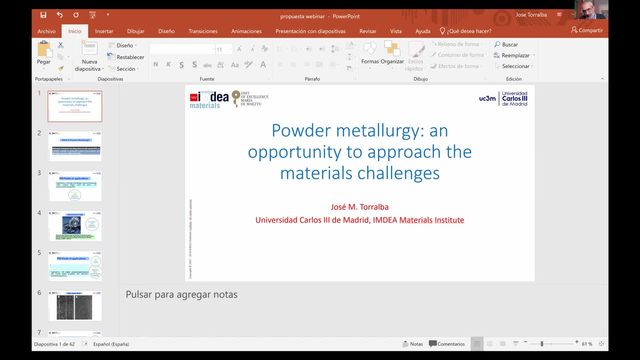 My companies start to produce big ingots of hot isototic pressing material. What we are trying to do in the industry now is to upscale at big scale the spartoplasma scintillating in order to have big blanks that can be machined. 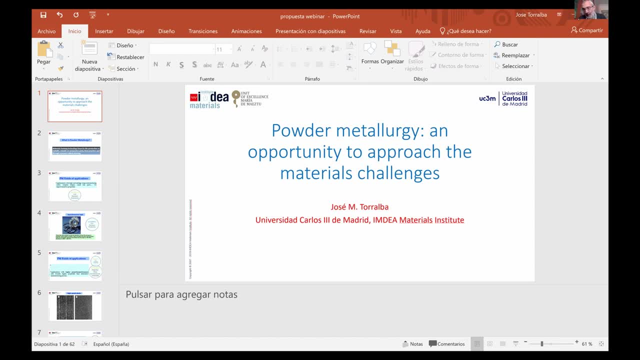 And in that case, now in Spain we have even one, the larger spartoplasma scintillating machine, which is in Oviedo, in one center related to the Institute of Caramel, which is Nanocare, which is a spin-off company. 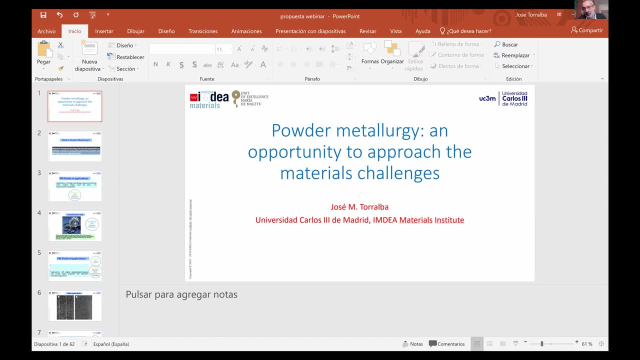 They have The largest spartoplasma scintillating machine in Europe And they can produce really big blanks that can be machined and used by some specific applications. Yeah, OK, So I don't know if there is any other questions. 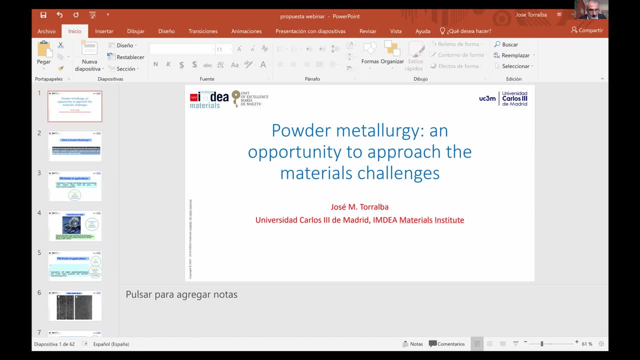 I'm looking at the chat to see if there is any more questions. Well, if not, I had another last one question. Is that, in your opinion, José Manuel, what do you think are the barriers that nowadays have the additive manufacturing technologies to be fully? 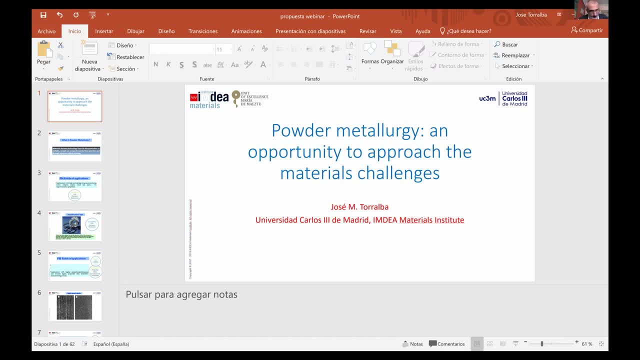 implemented in industry nowadays, Or the barriers, the what? Well, OK, One of the main barriers in some way is the powder development. The key point here is the powder. If you don't have good powders to develop materials. 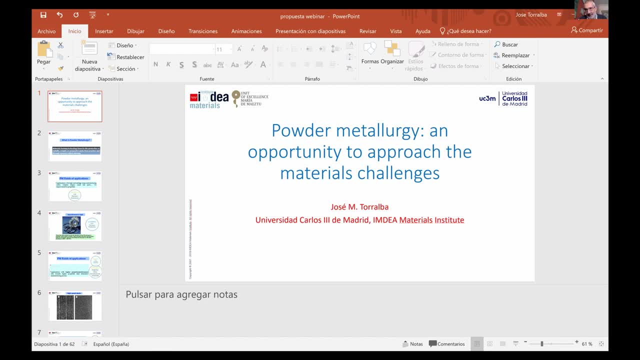 to develop parts, you have a problem. Yeah, There's an important barrier there. Fortunately, there are now a lot of new powder manufacturers that are involved in developing the new powder, fully powdered powders, especially fully powdered powders for the technology. 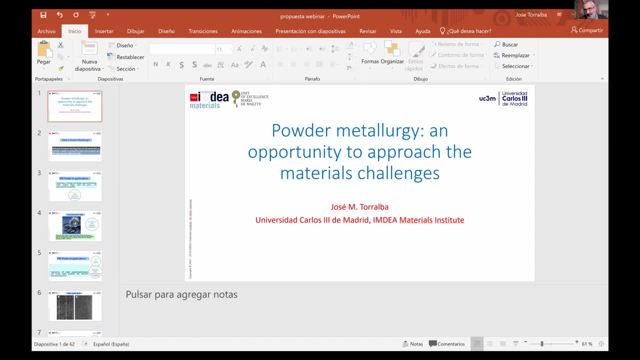 This is one of the barriers. The second one is the knowledge. I think there are a lot that even today there are a lot of people who is trying to go inside this technology without knowledge at all about the powder technology, And powder is the key point in the good development. 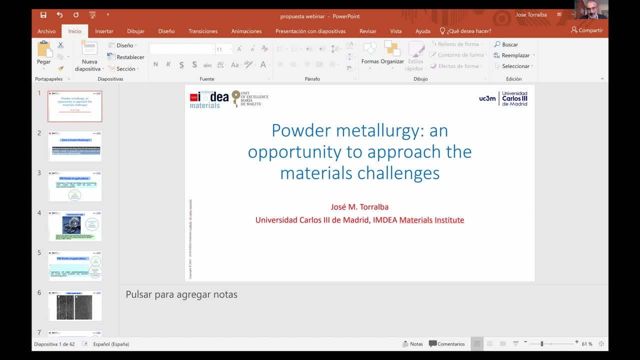 of the final part And by editing manufacturing. Fortunately, this is a thing that is now. I think most of the people have this thing in mind, that they have to know very well the powder that we are using before to put in the machine anything inside the machine. 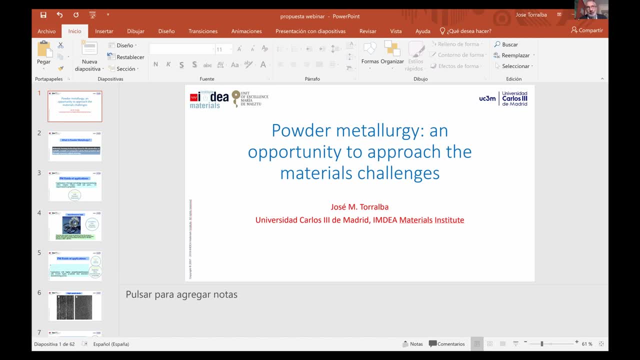 I think another important thing is to get knowledge about the process. The process has a lot of, let's say, weak points still now. So we have a lot of knowledge. We have a lot of knowledge to put inside the process, inside to solve the defects that we have when 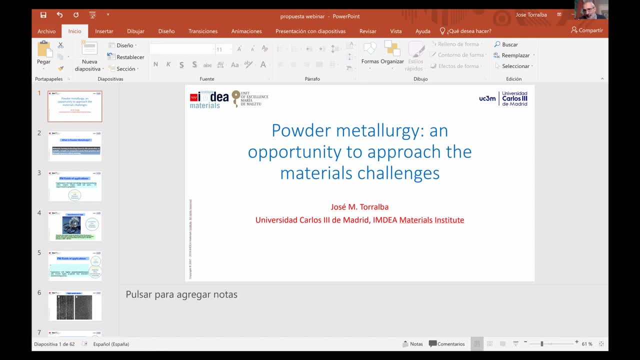 we are melting something in a very fast way, with a very fast cooling way, and so on. You have a lot of things in the process that could be improved. In that sense, the combination of the knowledge about physical metallurgy of the process and modeling 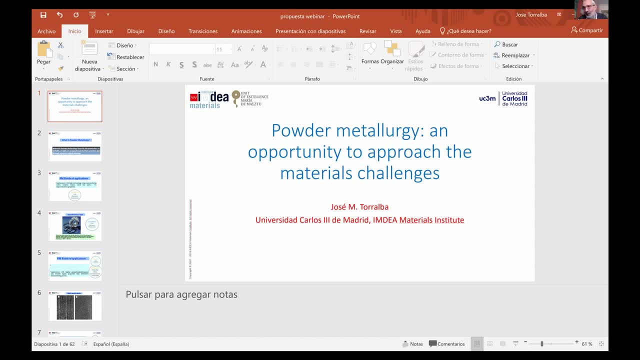 the modeling can add a good key factor here, Because by modeling we can advance a lot of knowledge, A lot of the problems that we can reach in the editing manufacturing machine. So this combination could be a good marriage in order to improve the properties. 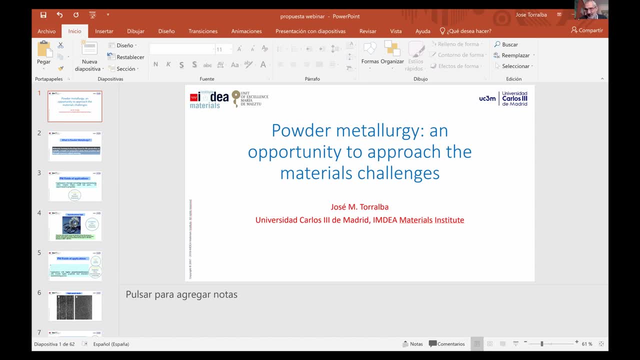 at the end of the editing manufacturing process. Yeah, I fully agree. Thank you very much. And very last question that some of the participants- one participant- made is what about the design of a specific alloys for additive manufacturing by CALFAT? 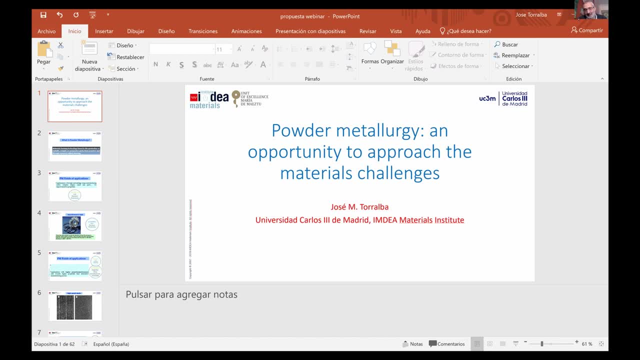 For sure, for sure. I mean today anyone can develop anything in material science without taking the advantage, taking the benefits of the thermodynamic, let's say, software that we have available in the market. So through CALFAT, through the thermodynamical method, 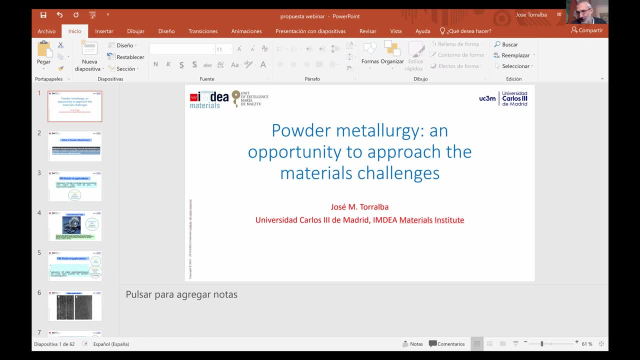 I think it's the first step to any development. So today it's unbelievable that anyone can use this, let's say tools- Yeah, Available- to develop any kind of new material. So in my opinion, this is the first step of any new research in material science today, in powder. 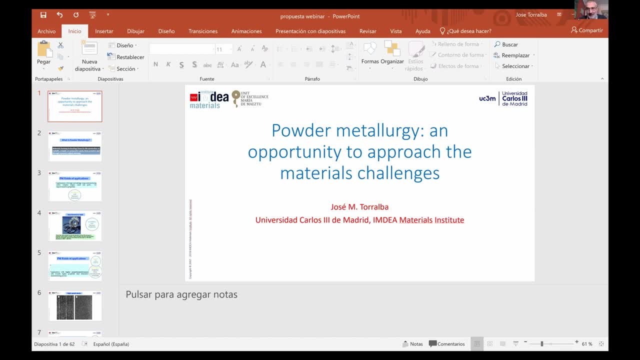 technology. Of course you can do the things by the old-style fashion way in which you can test the powders and trial and error you can reach a final design of material. But today, having CALFAT, having thermodynamical tools, 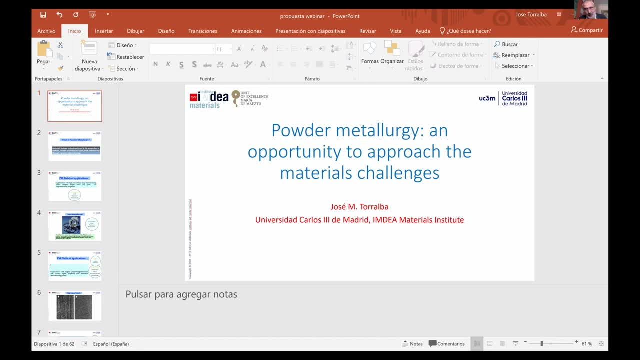 in order to develop the alloys. it's amazing that people don't use it, So I encourage to use these techniques to develop new materials. OK, so well, it's 1 o'clock now. There is one question. I think Rocio is talking on something. 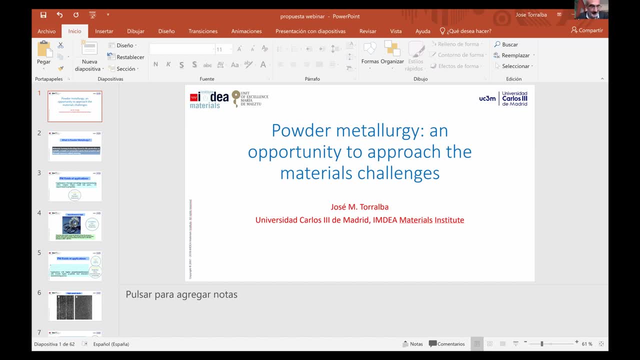 Rocio Munoz from HHPA regarding the binder jetting technologies. I think, regarding the sintering in binder jet, I have mentioned before that sintering is one of the key parts of the development Because, at the end, after printing the material, 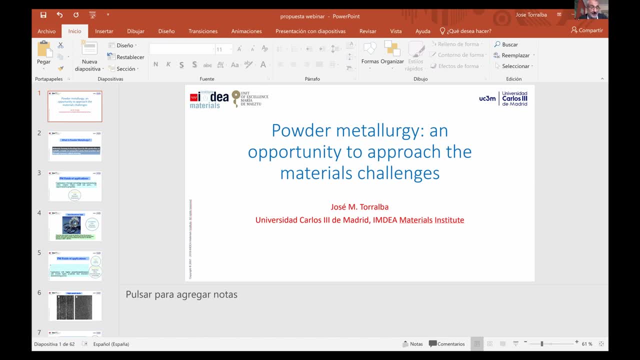 after print the material, at the end you have to sinter the material. So the combination of powder metallurgy, the conventional knowledge in powder metallurgy about sintering techniques and sintering process, and the printing, which is the in that case. 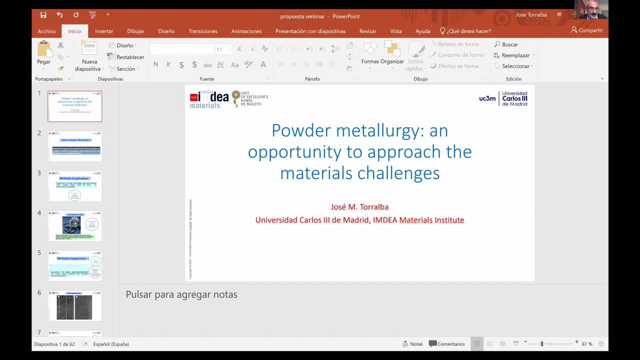 the special know-how that they have in fellow packer. I think it's a good combination, also in order to try to develop much better the material. Yeah, I think also she was trying to clarify a question regarding What do you mean by HP method. 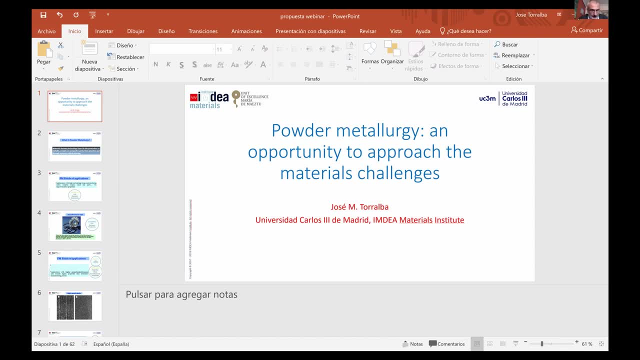 And she was just clarifying through the chat that HP is a binder jetting based technology, metal jet HP technology. So she was basically clarifying this to another attendee. OK, so well, thank you very much. I don't think we have more time. 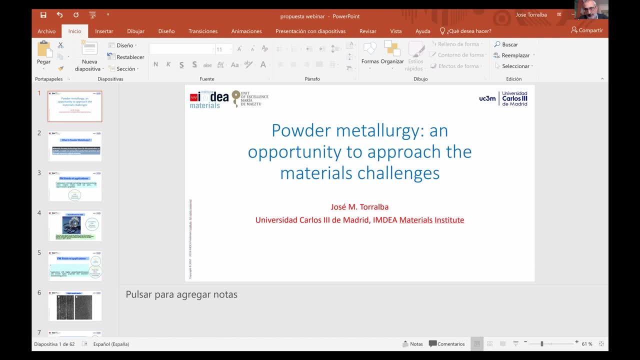 And this is 1 o'clock. Well, Jose Munoz, thank you very much for this webinar. I think it was a very, very illustrating, very, very inspiring, And I think at least you gave an overview of the different possibilities of powder metallurgy. 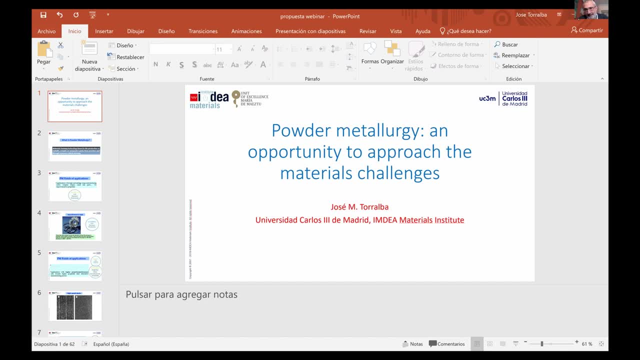 And if anyone would like to get further information, please contact Professor Torralba directly. You can find all the contact details through the web page of India Materials or the Carlos Tercero University. And well, as I said, this is the first webinar. 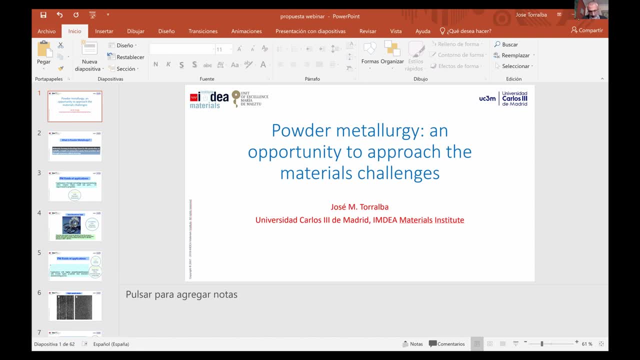 Many other seminars will come soon from India, Materials And well. with this, I wish you that all of you and your families keep healthy And well. thank you very much to everyone And thank you very much Jose Manuel. Thank you. 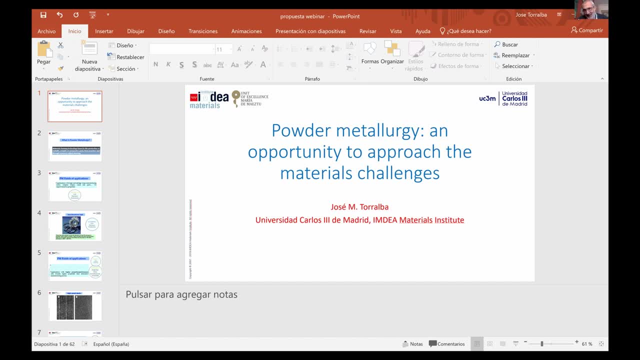 Let me just to say thank you to everybody to be so patient with me, especially to those people who are experts in powder metallurgy- that maybe some of the things that I have been talking about are well known for all of them, But I have tried to make a lecture open to everyone.